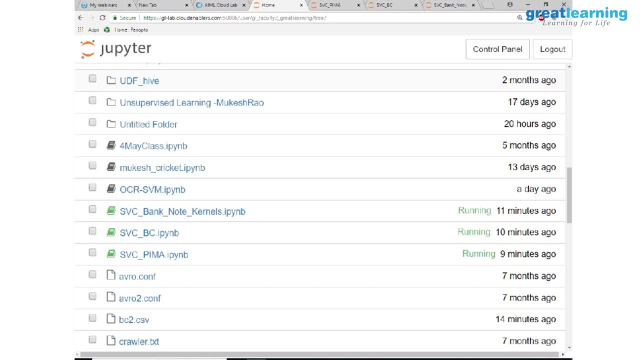 on both sides when you have maximum margins on both sides. the maximum margins are called no man's land. none of the data points from either class should be inside. that is called hard margins. When you take this model to production, very likely it is going to perform lesser errors. 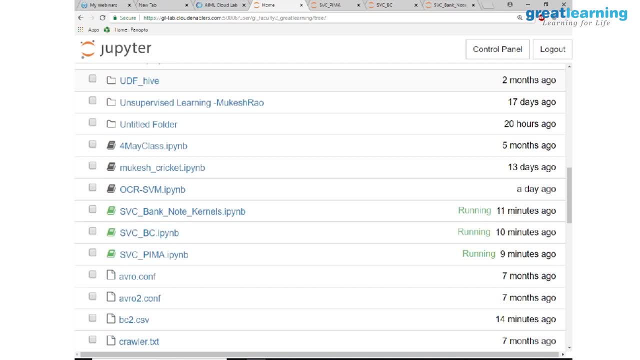 relative to perceptron in production. To be able to achieve this, you need two things. one, you need to be able to find out the distance of a data point from the line, and the second thing you need is you need to be able to compare the lines to. 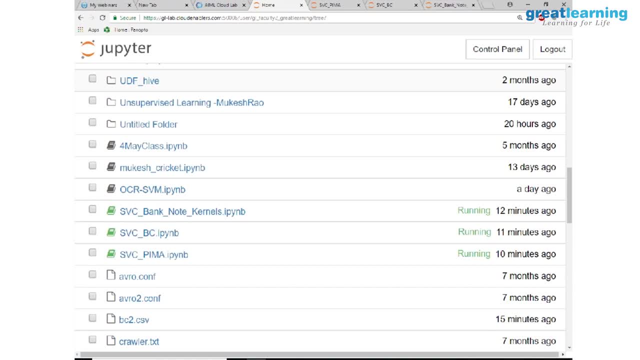 find out which is the best fit line. So you need a way of comparing the planes from one another, then you need a way of finding how far away a point is from a line. If you have these two ways of measuring, then you will be able to find out the best fit. 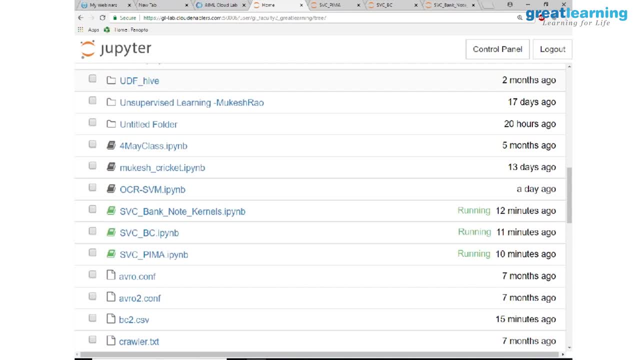 line. Now, what I have done is I have taken some of what you call some fictitious numbers, on which I have done some calculations, so I am going to show that to you here. First of all, do you know what is? how do we represent a line or a plane? 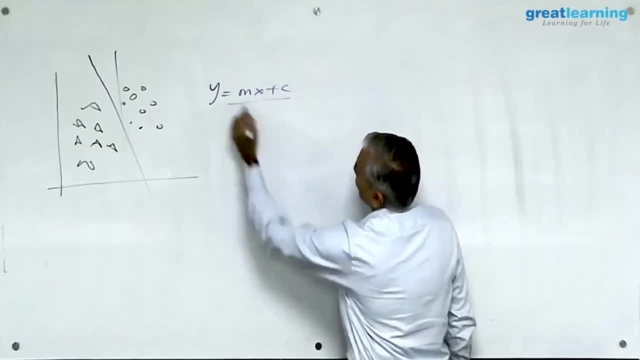 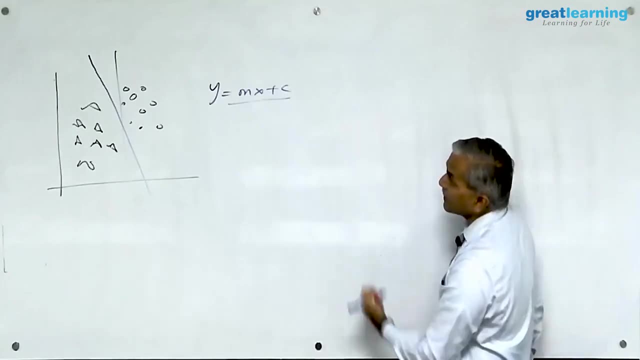 All of you are familiar with this right. Anybody who is not, do not hesitate to say no if you are not. Now, this is what we have been taught in school: that y equals mx plus c. but the way you can express a line as an equation. 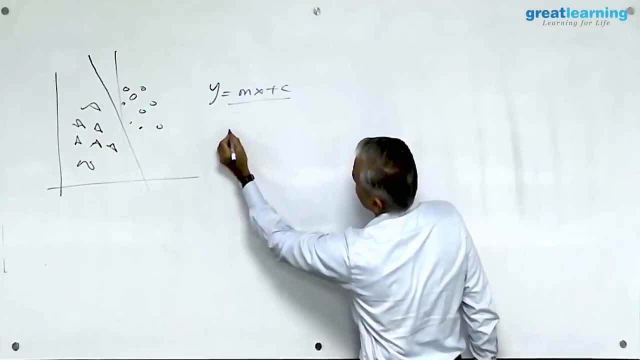 You can treat this as a variable, So I can call this: for example: x2 is equal to mx1 plus c. 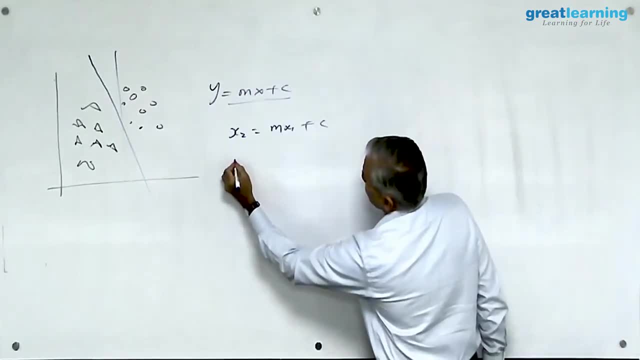 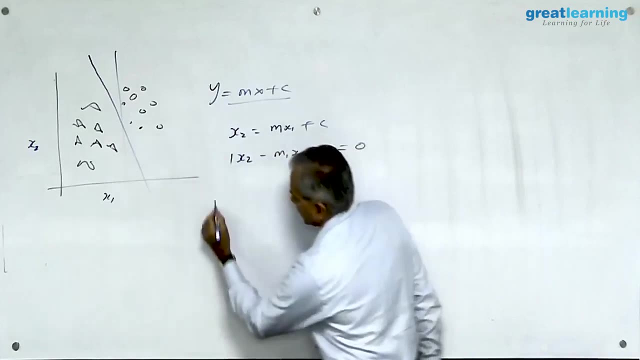 Any problems? No. So I can also write this as say: 1 more x2 minus m1 through x1 minus c is equal to 0, because, lying when you look at it, a line has not only slope on x1, it also has a slope. 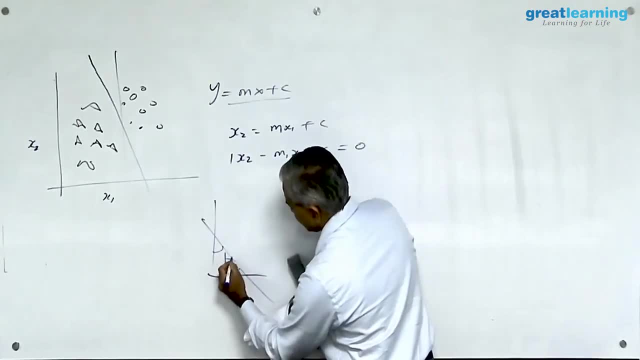 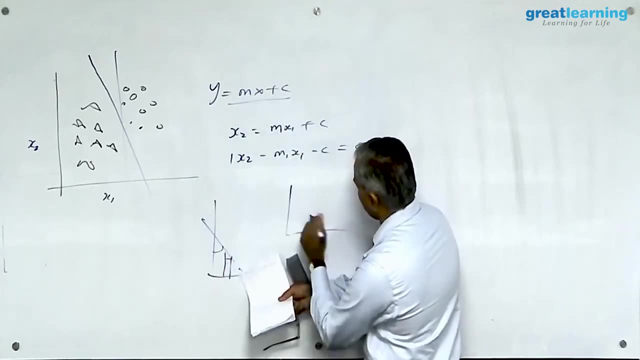 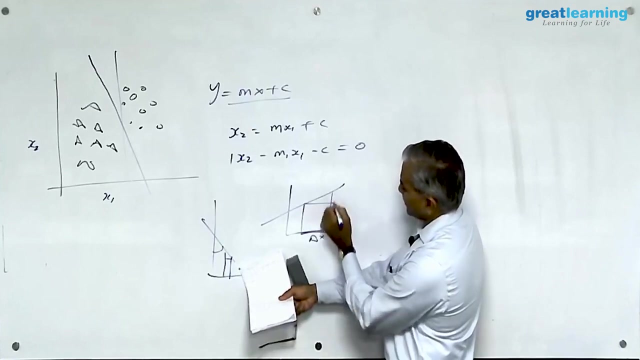 on x2.. Slope is dy divided by dx is how much y changes for every linear unit change x. So this angle, this angle, I will draw it bigger. Suppose I write it like this: This is my dx: How much your y changes for a given dx dy. this ratio is called slope. 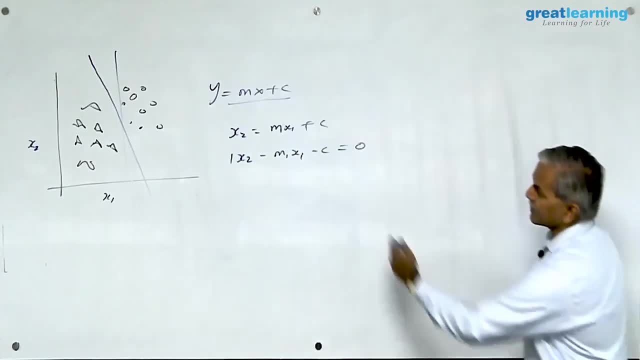 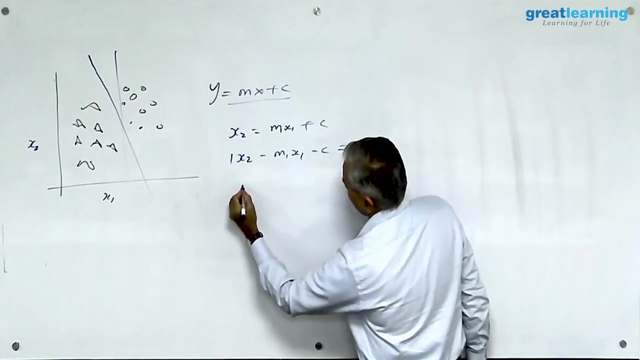 The tan of this angle is slope. So I can express the equation like this: Basically, equation is being expressed in form of both these coordinates. Now let me take so this: what is this? shown to you? as is equation line can be shown as w, comma b, where w is. 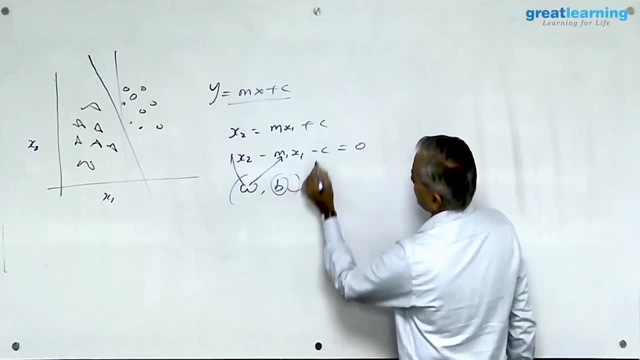 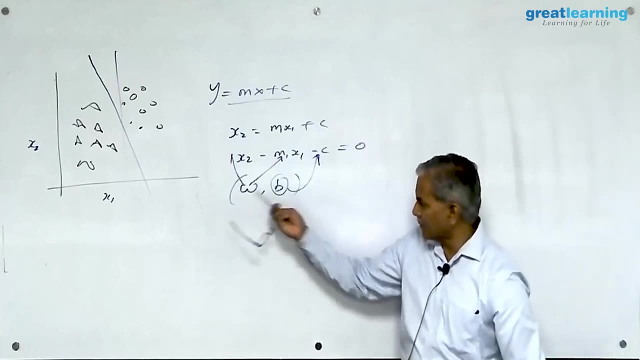 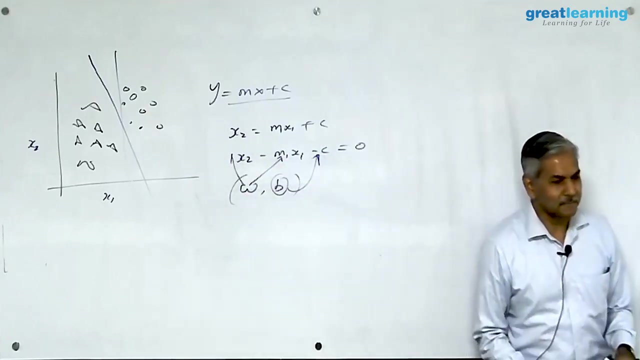 the weights given to these two, and b is your constant. You will often come across books in which they will say the equation of line, they will represent it by w and b, where w is nothing but these two. So these two, these two coefficients, this one and this one, and b is the constant. These 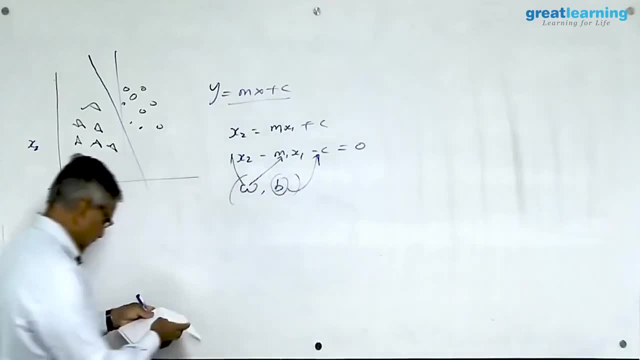 are different ways of showing things. It does not make any difference, But please tell me whether you are ok with this. So in this, our case, in this example which I have taken, w is a list of two values, 1 and m. b is nothing but your c. 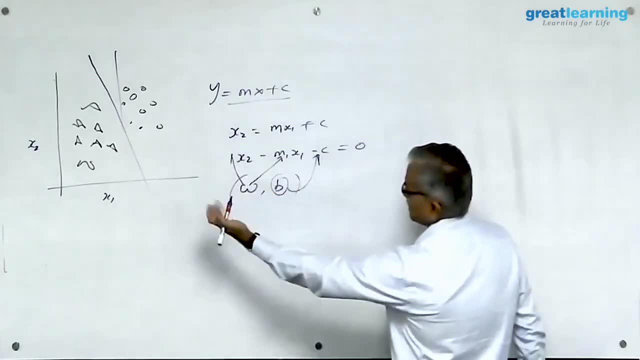 So what I have done here is for explaining the concepts. I have taken a value of a- w is. I have taken a value of m and from a value of a I have taken w as m, And now I have: 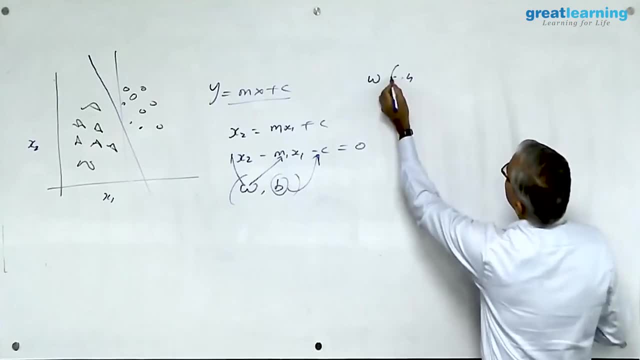 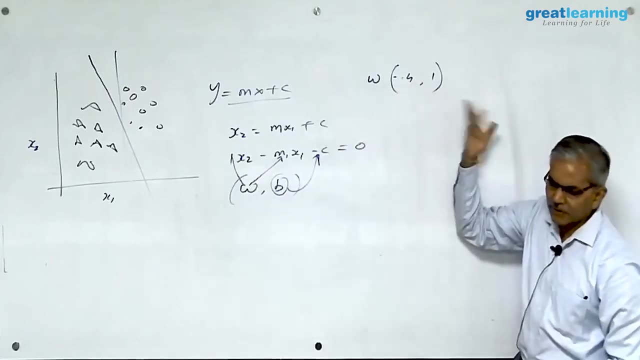 taken a value of 0.4, some randomly picked up numbers, and this one is 1.. I have just taken these two values minus of 0.4 and 1.. You can ask me why? no reason You can take. 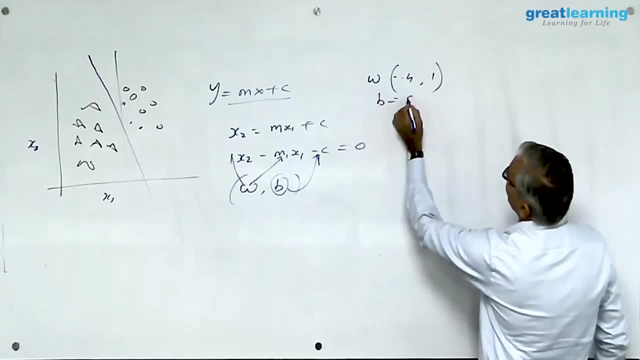 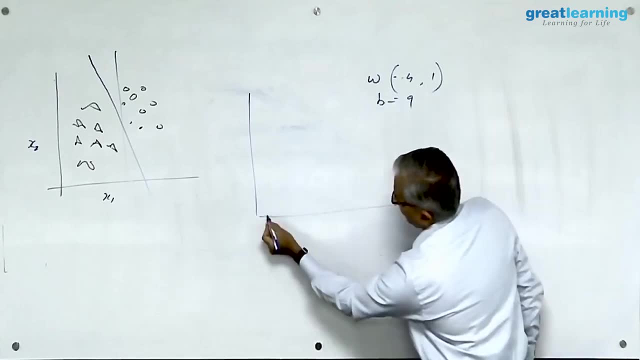 any other value And the b. I have taken it as 9.. Once again, no reason. you can choose any number you like, So let me draw this now. You have 1,, 2,, 3,, 4,, 5,, 6,, 7, 8.. I will show. 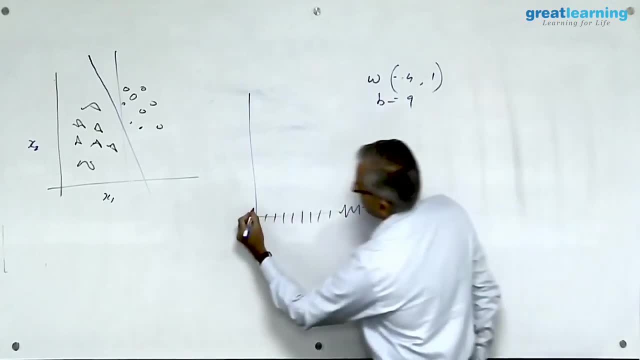 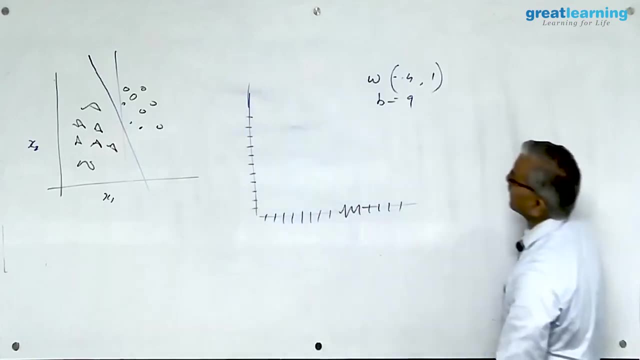 you a kink, then so on, so forth. Then this side, you have 1,, 2,, 3,, 4,, 5,, 6,, 7,, 8,, 9,, 10.. It goes up. Now look at this equation that you get out of this, The equation which comes: 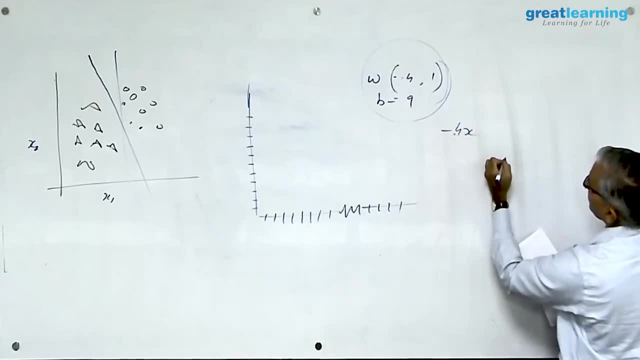 out of this is minus 0.4 x x 2, right, And this x 2 minus 9 is 0, means x 2 becomes x 2 becomes 9.. If minus x 2 is: 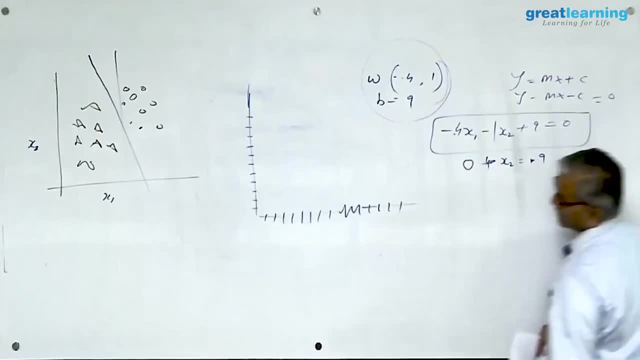 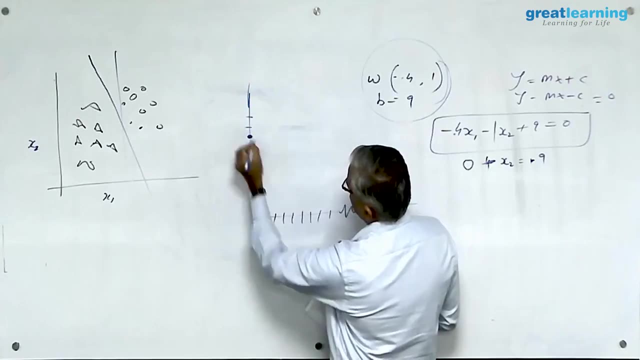 minus 9,, then x 2 is 9, okay, That means when x 1 is 0,. x 2 is 1, 2,, 3,, 4,, 5,, 6,, 7,, 8,, 9.. 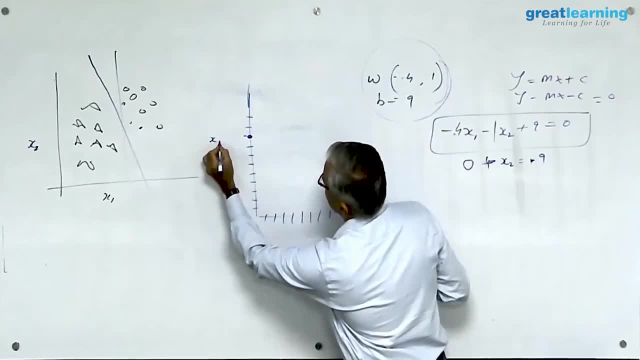 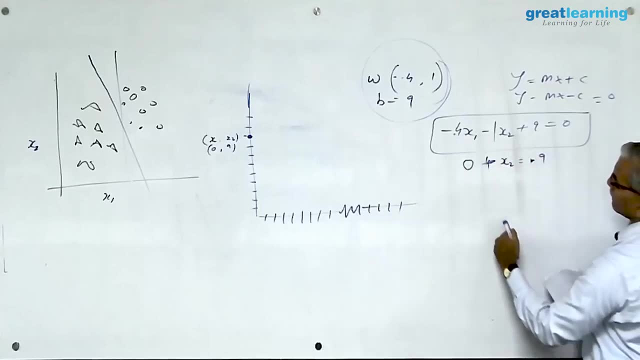 This is the point where you have x 1 is x 1 comma x 2, this is 0 comma 9.. Let us take it other way round. When x 2 is 0, minus 0.4, x 1 is equal to minus 9 or x 1 is equal to. 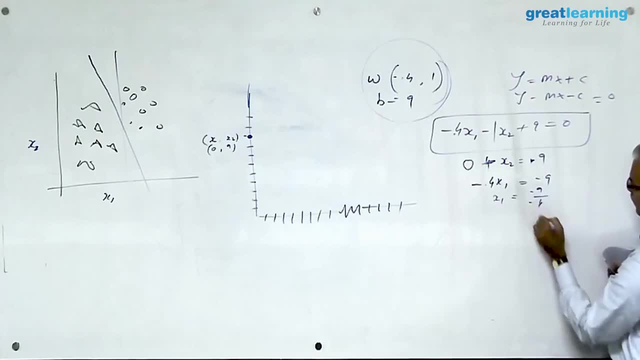 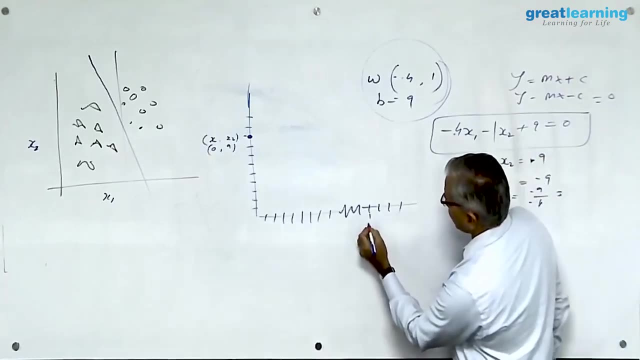 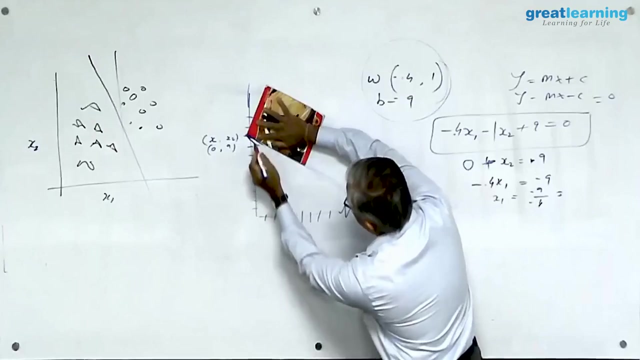 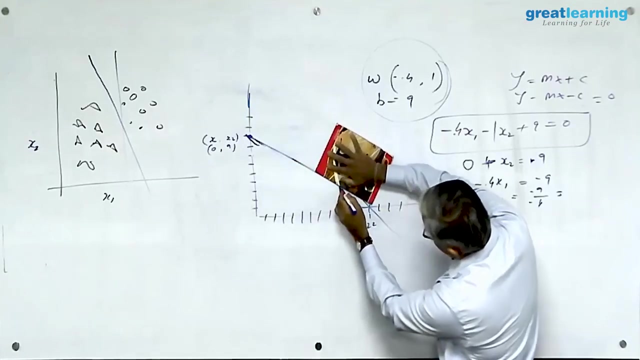 minus 9 by 0.4,. this will come to 22 something. okay, Okay, 2.25? 22 point something. it will come right. So let us assume that 22 is this one. It is too long, right? So we draw a line from here. Let us put the straight line here. Suppose, 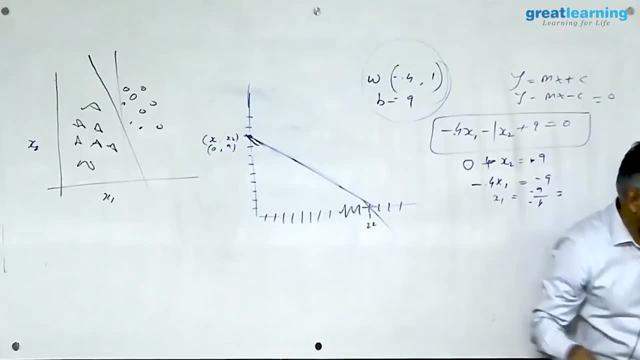 this is 22.. All of you, okay, This equation, this line, is what is equation by this surface? Okay, Now the. how do you find the distance between a point and a line? Again, without going into mathematics, what I am going to do is, I am going to take three points: The: 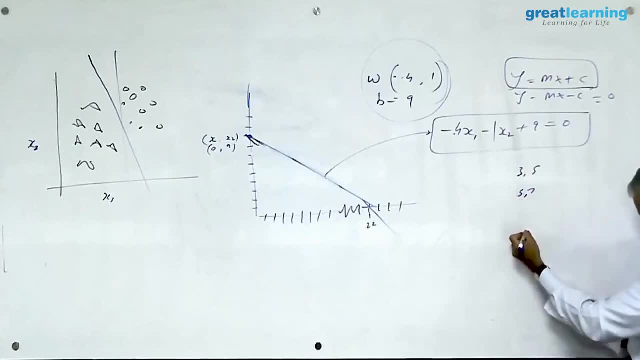 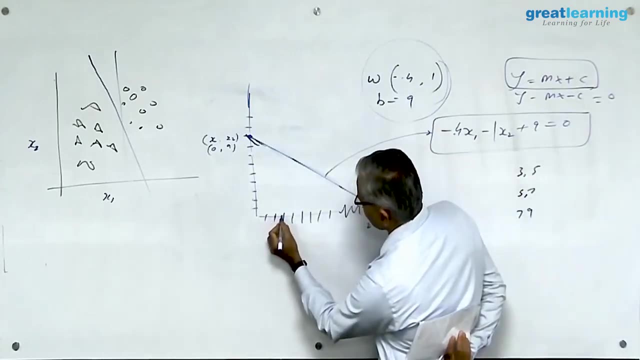 points I have taken are 3, 5,, 5, 7 and 7, 9.. I have taken three points. Let us take the 3 and 5, okay, I hope it comes out right. 1, 2, 3, this is 3 and 1, 2, 3,, 4, 5, this. is 5.. The place where they meet: this is the point Okay. 1,, 2,, 3,, 4,, 5, this is 5.. The place where they meet: this is the point Okay. Now let's. 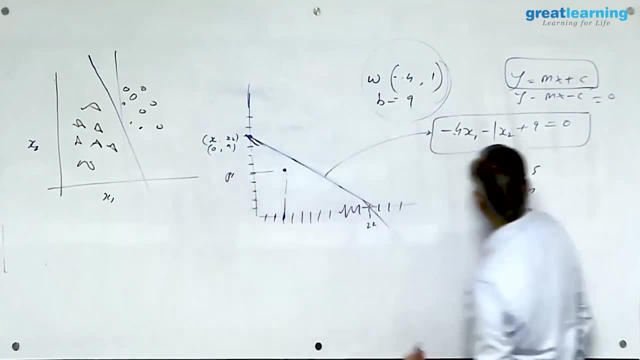 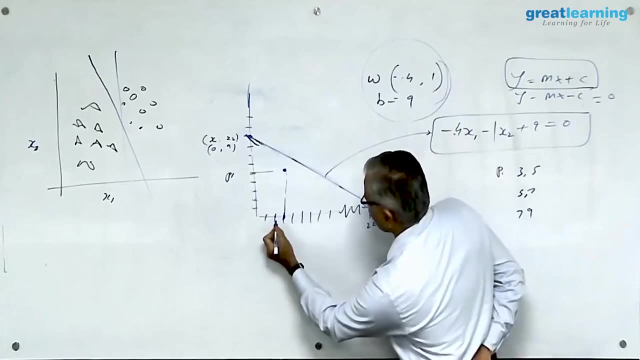 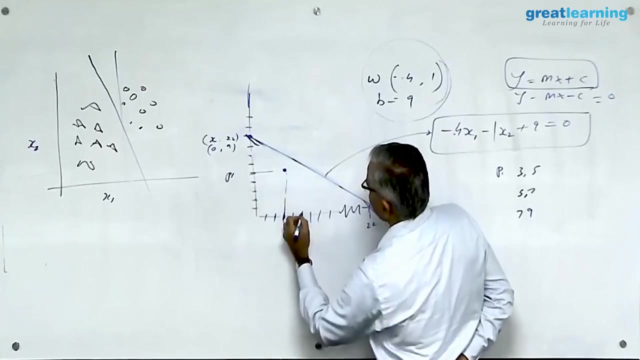 point. This point is P 1, where P 1 is 3, 5.. Take the next one: 5, 7,. I really hope 1, 2,, 3,, 4, 1,, 2,, 3,, 4,, 5,, 5 and 7, 1,, 2,, 3,, 4,, 5,, 6, 7, 5 and 7 are supposed to meet. 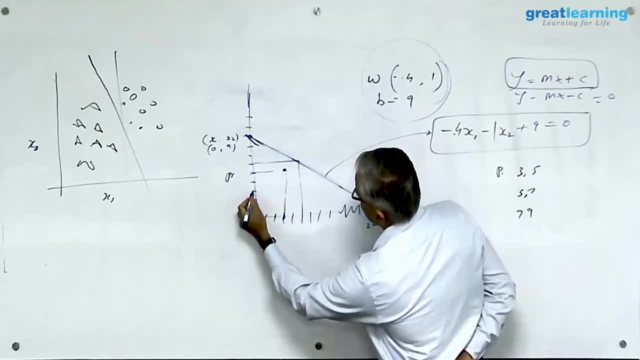 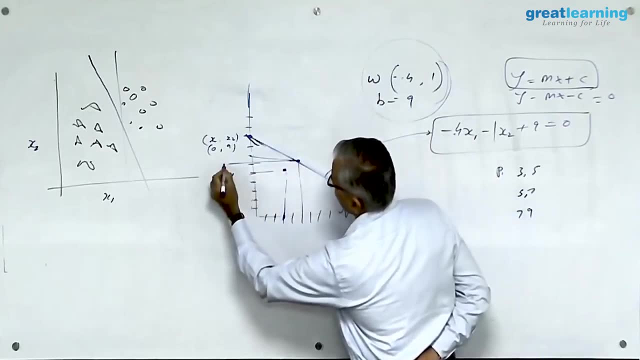 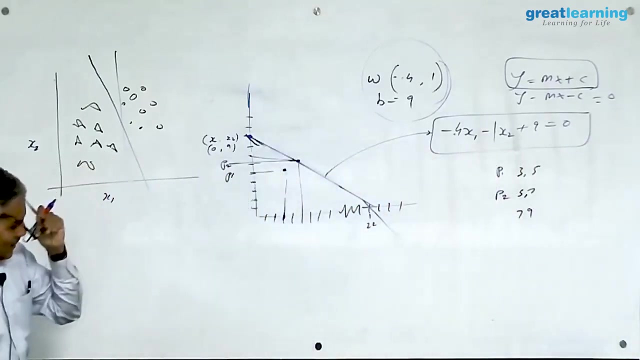 on the line and suppose they meet on the line 1,, 2,, 3,, 4,, 5,, 6,, 7, oops, suppose it is going like this. This is my P 2.. This point is P 2.. Are you ok? all of you. Similarly, the. 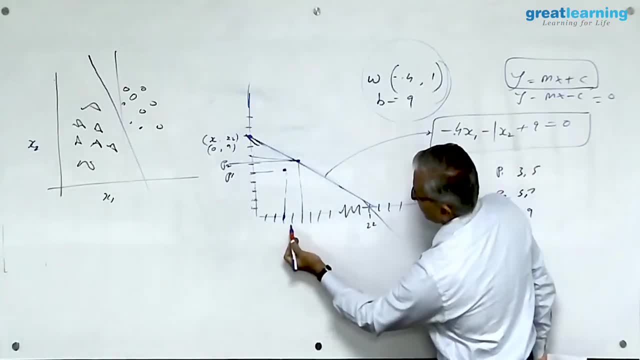 third point is 7, 9.. So 7, 9 comes to 1,, 2,, 3,, 4,, 5, 6, 7 and 9 is 1,, 2,, 3,, 4,, 5, 6,. 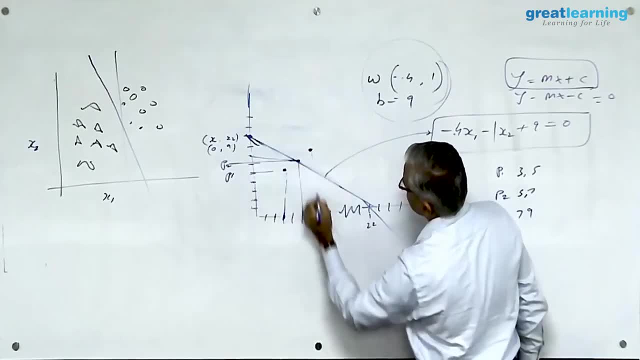 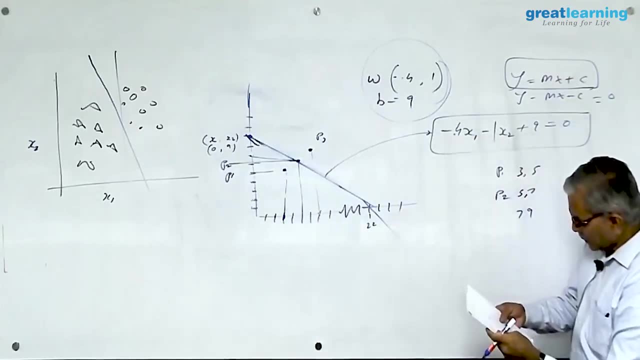 somewhere here, 7,, 9, ok, somewhere here. This is my P 3.. All of you do one thing for me, please. What you have to do is you have to, you have to submit these, substitute, these values into this equation. Will you please substitute? 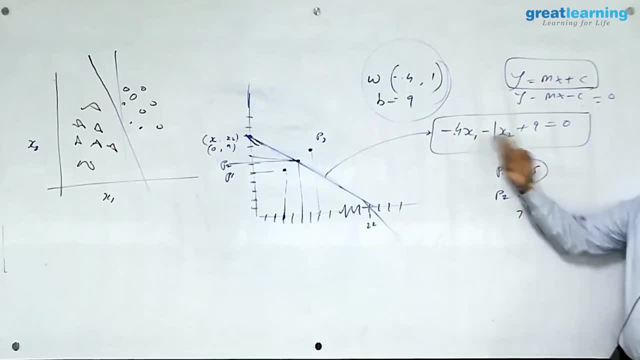 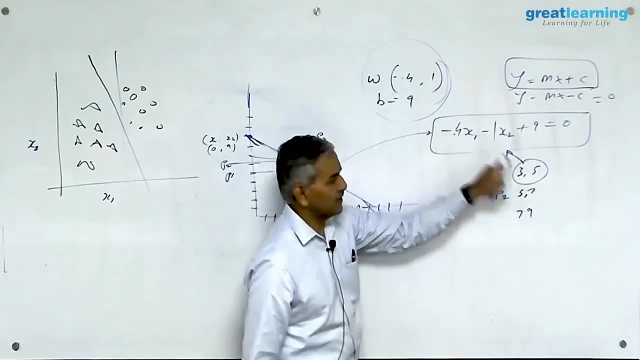 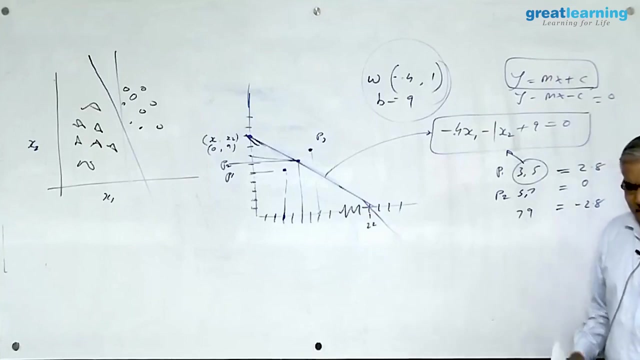 these values into this equation for x 1 and x 2 and tell me what you get. Just substitute these equations into this equation, these values, and tell me what you get. First one is 2.8, minus 2.8.. I have consciously, I have deliberately taken these points. 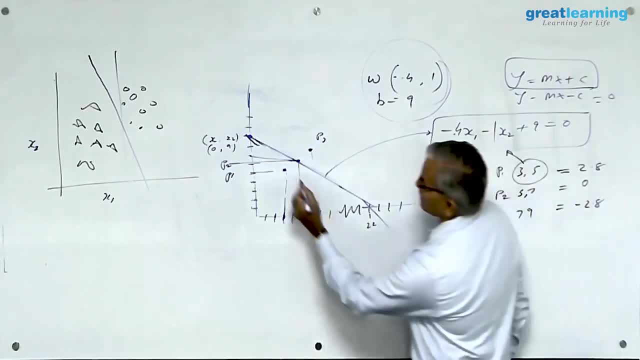 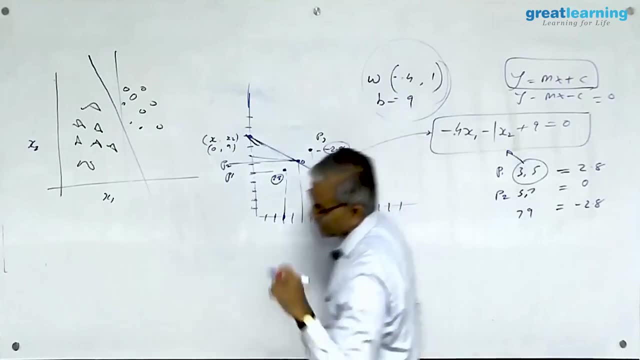 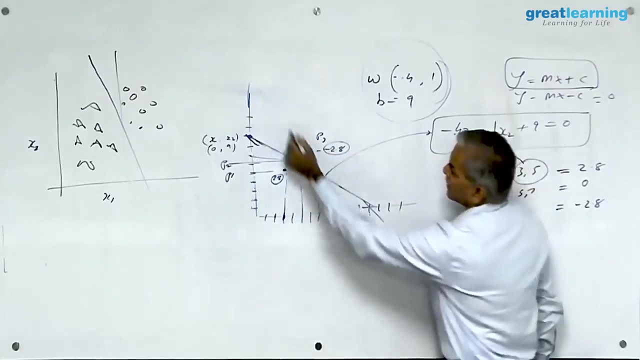 To get exactly same number. Ok, This number is 2.8, this number is 0 and this number is minus 2.8.. That is what you will get Now when I give you a distribution of points and there are various planes like this: various. 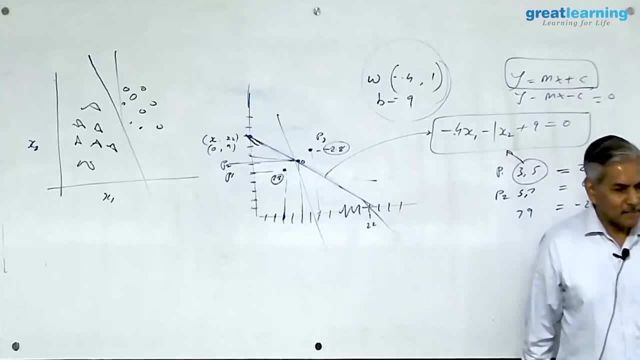 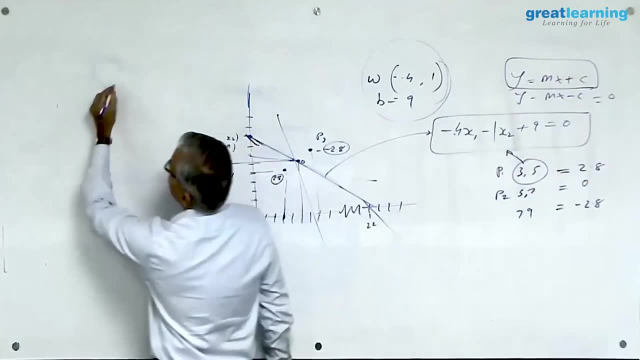 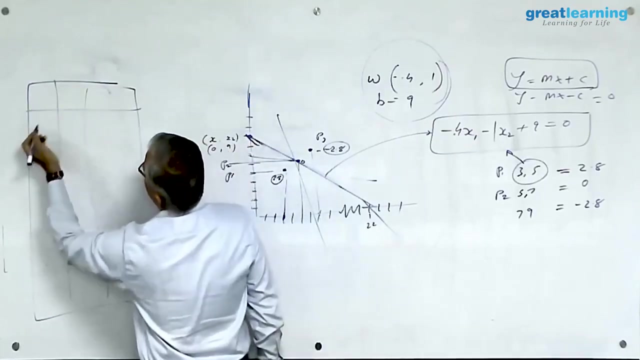 plains, cutting in the mathematical space for every plane, every plane, I can find out the distance of the different points from those planes. Suppose we create a table and in the table there are three columns. The first column is your w, the x1, y1 and 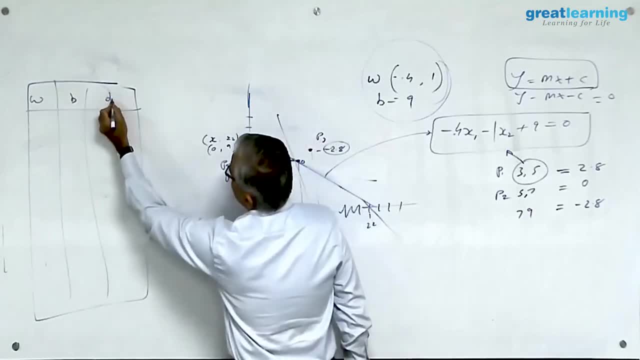 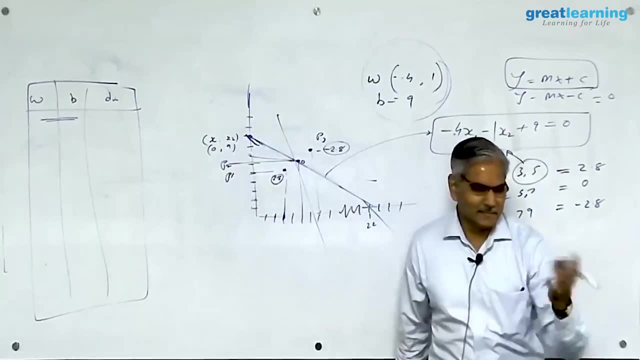 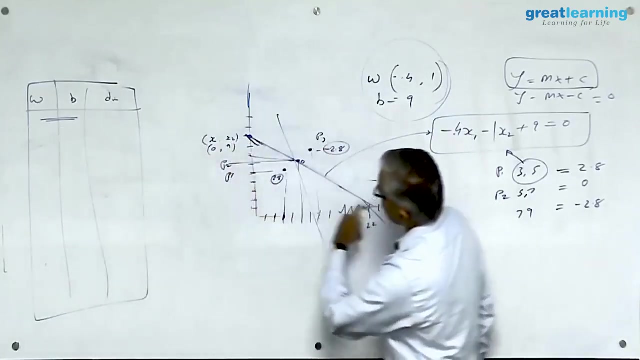 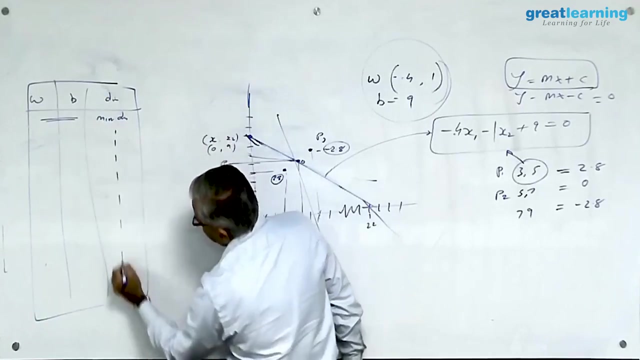 the next column is your b, and then you have the distance. For every combination of w and b you get a different line, different line. So for every line or model you find out what is the minimum distance point, You find out the minimum distance, min-dist- for every line. 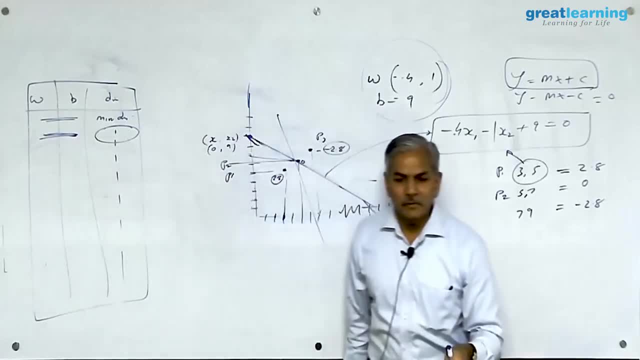 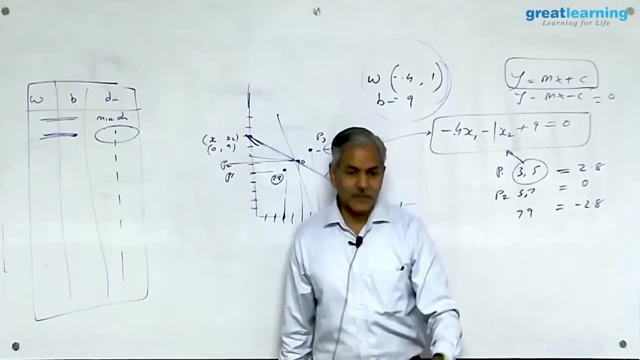 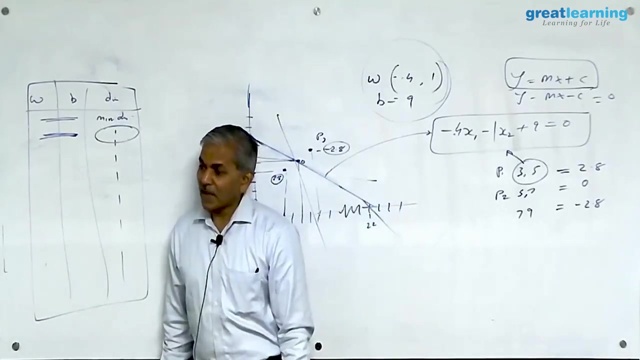 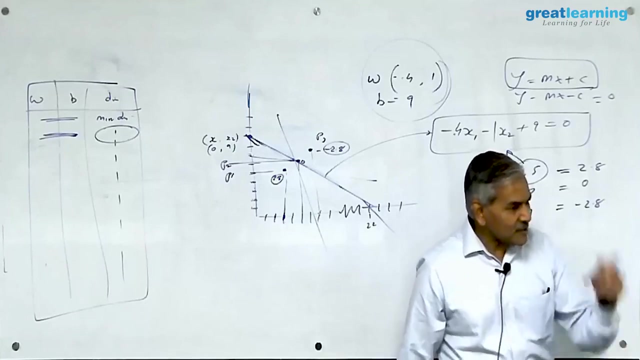 That combination of line. that combination will give you the best fit line, The line which is maximally the maximum of the minimum separation. that line will be your best fit line. Maximum of the minima. Find the minimum separations for all the planes Out of that. pick up that plane which has: 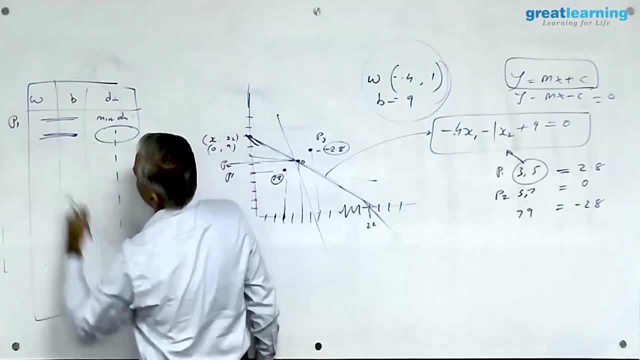 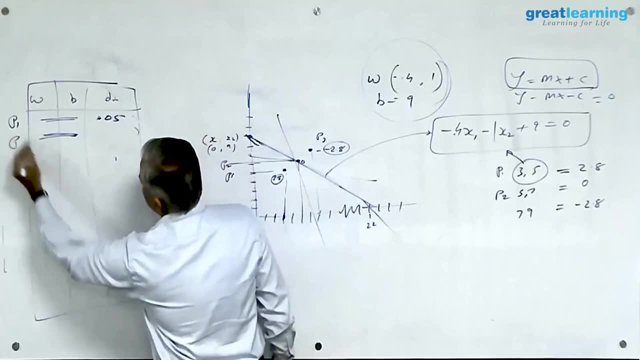 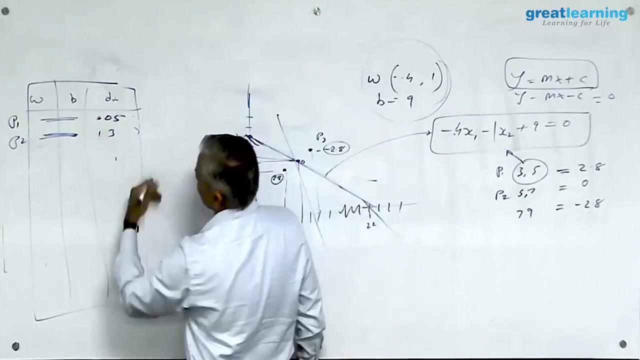 maximum value. Suppose you have taken plane 1, p1 and the minimum distance of this p1 is 0.05 something. Then you take p2, p2- minimum distance between any data point in p2, the minimum distance is, say, 1.3, something of that sort. You take p3, 0.5, go on, pn, whatever. 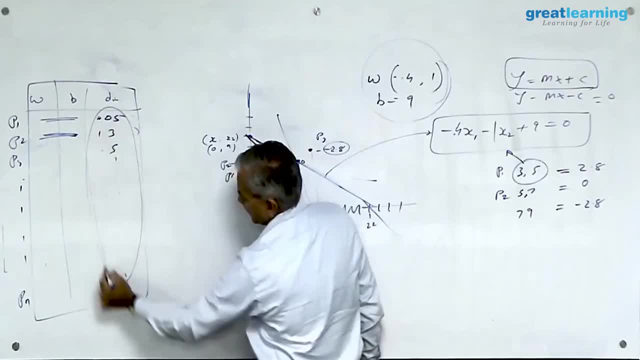 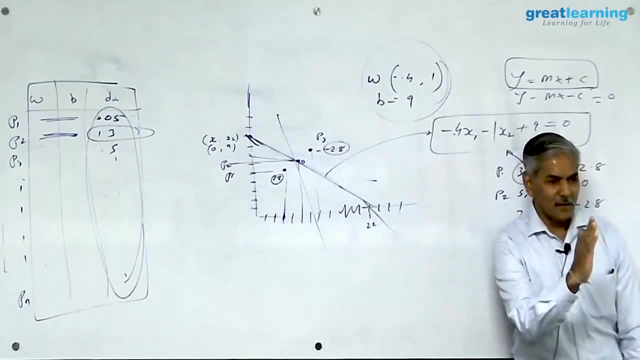 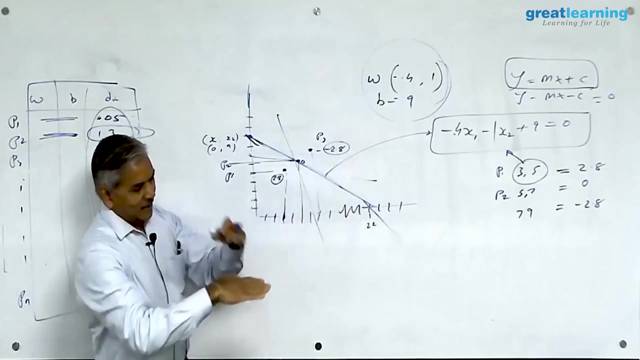 the value is. These values, take the one which is largest. This is the plane which is maximally separated from the data point from the two sides, And for every combination of slope and constant you get a line. Find out which is the point in the mathematical space which is closest. 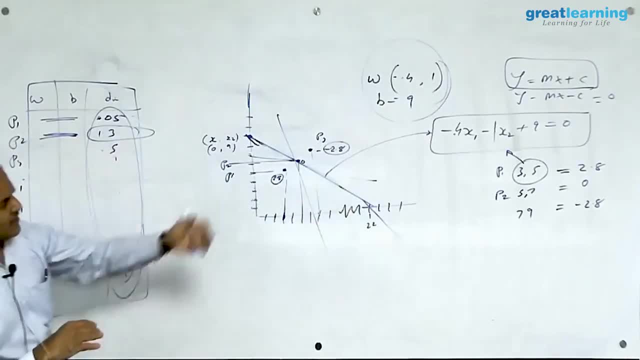 to this line. and what is the distance? How do you do that? Just substitute the position of the point into the equation, So you will get the distance of the point which is closest to the plane in a mathematical space. So from this list you take the one which is highest, So this plane is the plane. 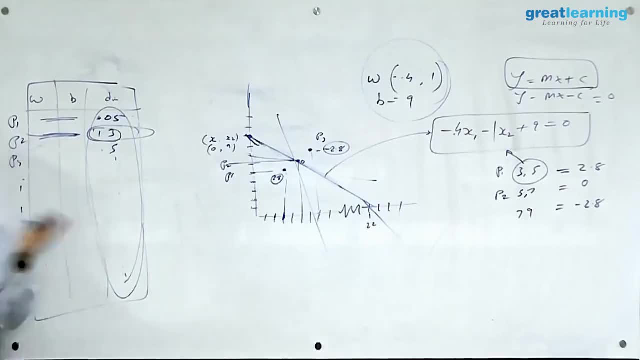 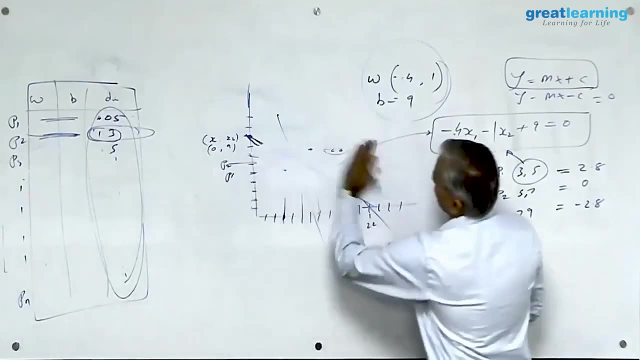 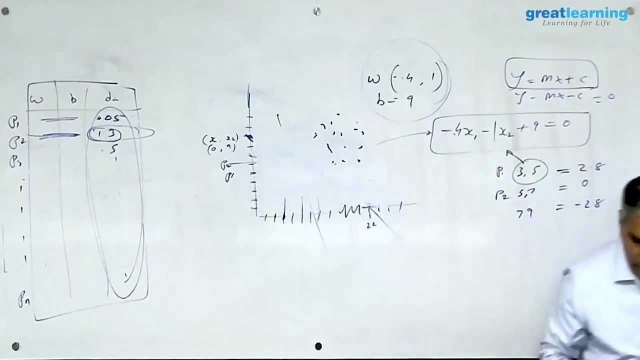 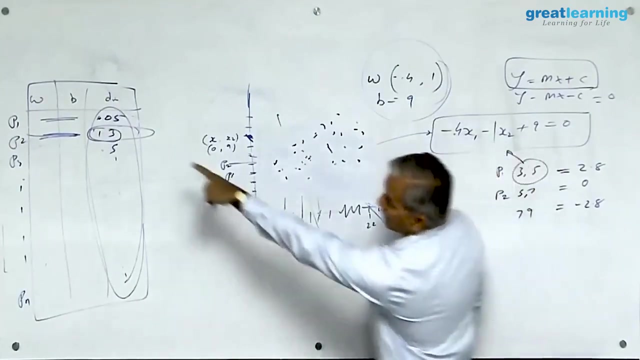 which goes farthest, I mean has maximum margin on both sides from the classes. So if my, if look at this, We have data points here from one class. You have data points from this class. You have data points here from the other class. This is a black Now p1. 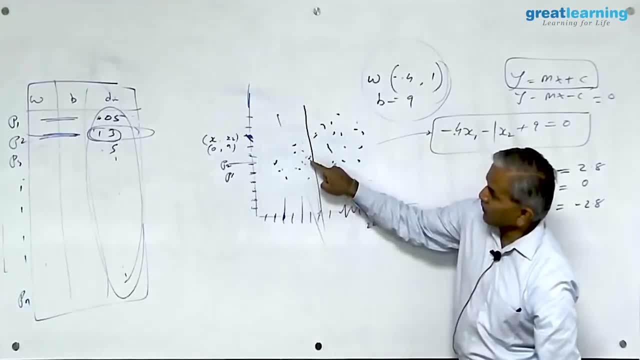 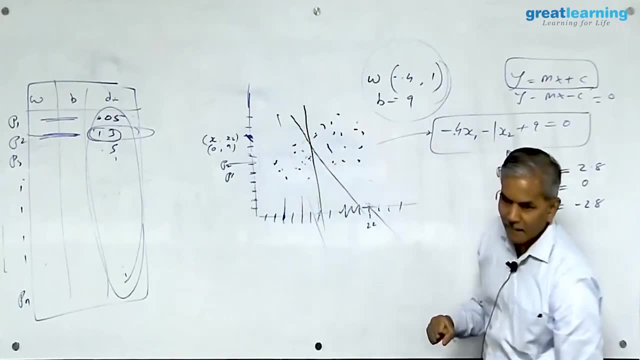 is this: It is going very close to one of the black points. So distance is this? p2 is slightly better. The closest data point for p2 is this class, This distance, is this what you reflected here? p3 is 0.4.. 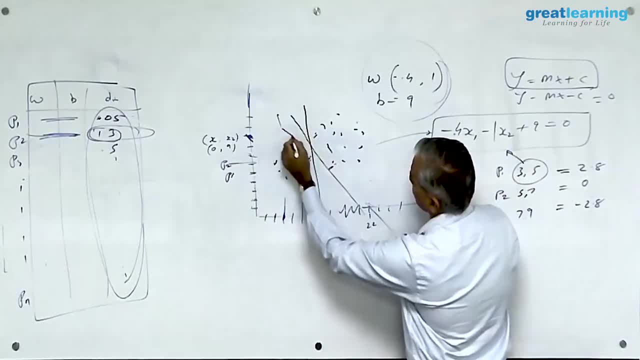 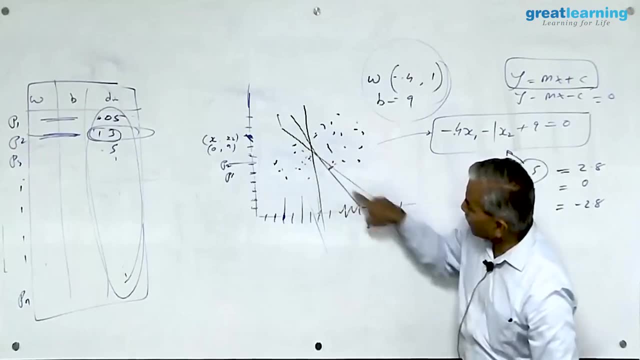 p2 is 0.4.. p2 is 0.4.. p2 is 0.5.. Maybe p3? you have drawn something like this. It is going very close to. I will compute. So for all these lines you find out the minimum distance between any data point in. 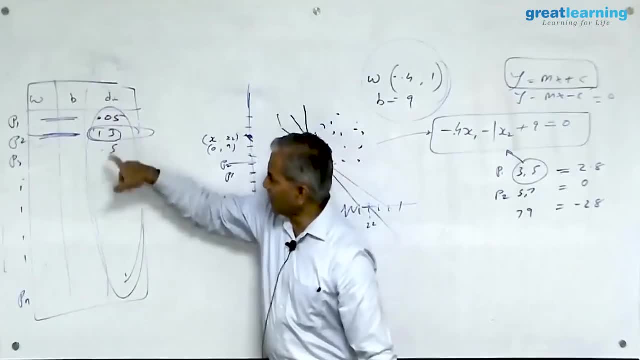 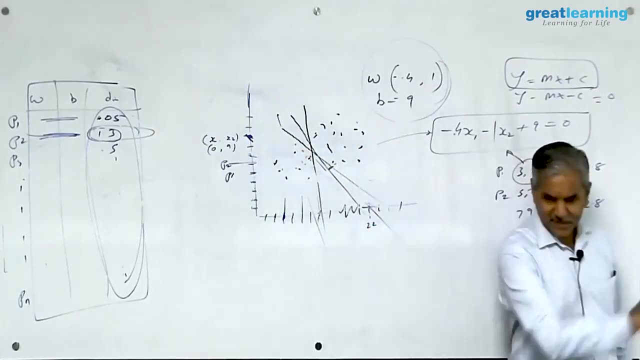 the line and put it here, Sort it and get the max. So the max is this one. This will be your best fit line. But there is a catch here. The catch is: points below the surface are positive. You saw it yourself. 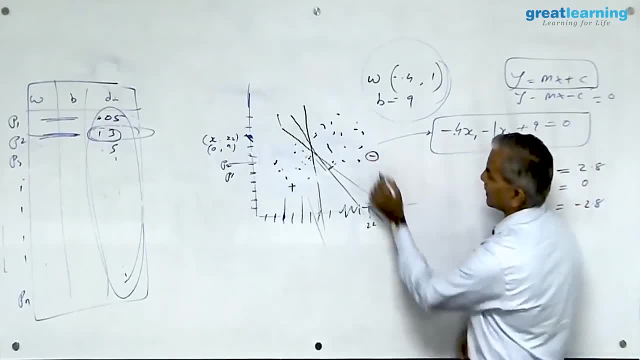 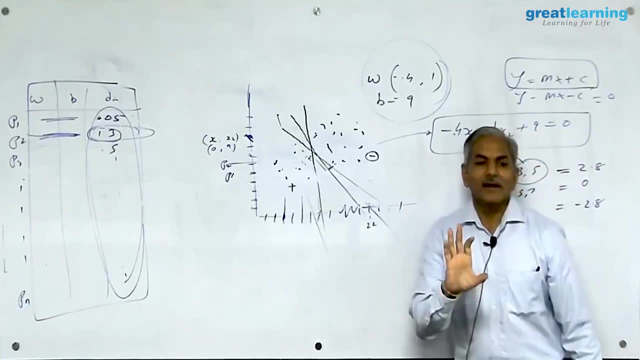 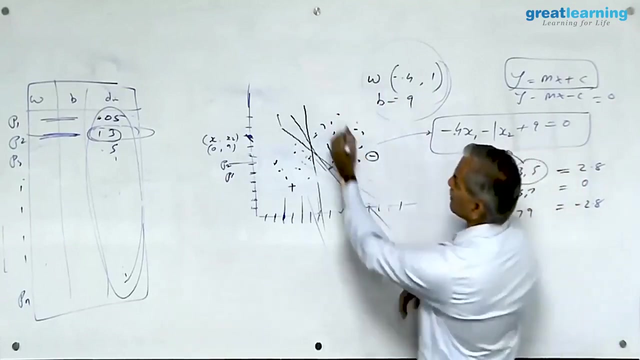 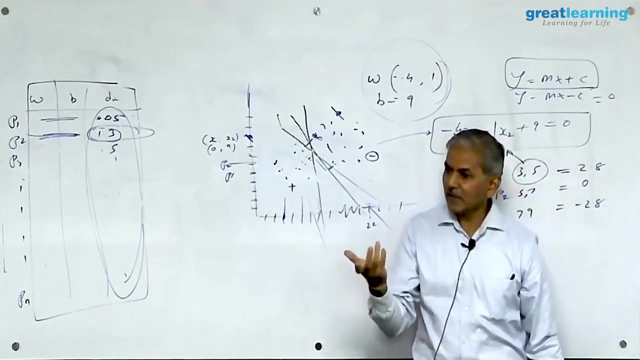 Points above the surface are negative. You want to find the least distance. When you want to find the least distance minus 1, a distance of minus 1 and a distance of minus 5. This will be minus 5.. This will be minus 1.. Which one will be taken? You are saying: 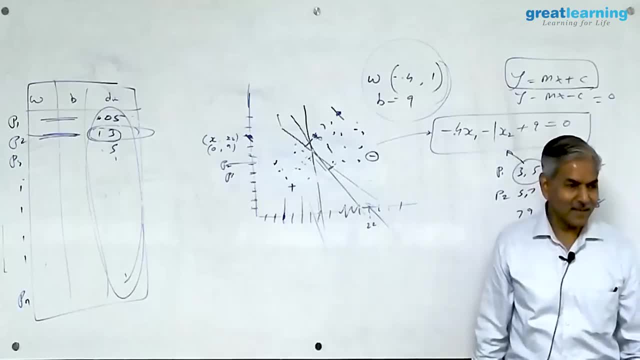 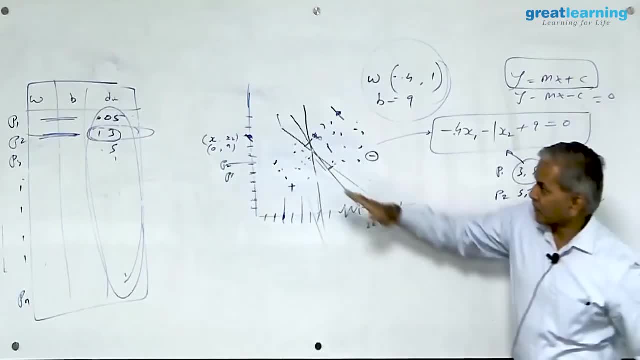 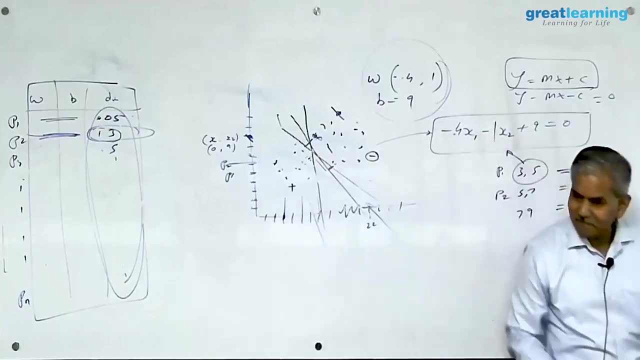 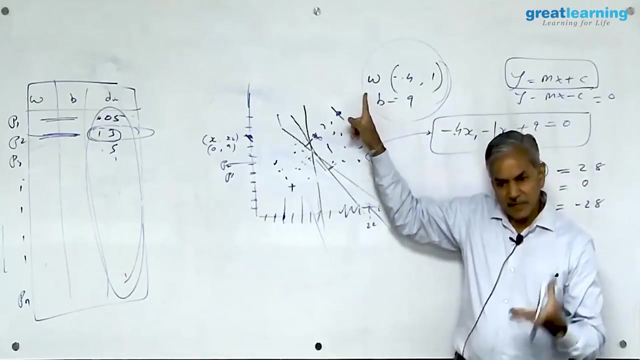 is the least distant point. But the problem with this is when you dichotomize your mathematical space using linear surface. one side gets minus, the other side gets plus plus sine. So when you talk about least distance, the largest magnitude negative value is the least. 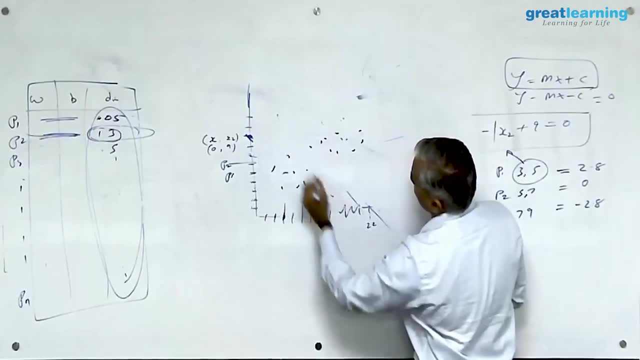 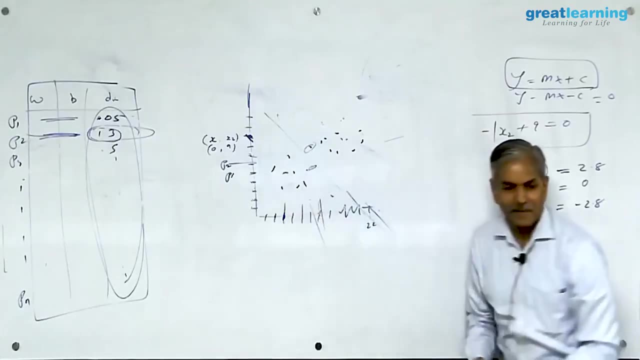 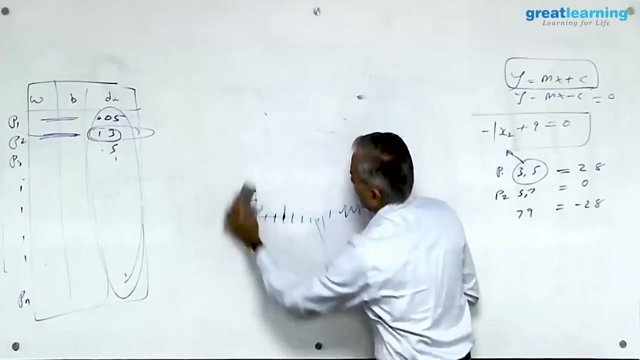 You look for the distance between the points, irrespective what sine it is. just look at the modulus, the magnitude- okay the magnitude- and find the best fit line. But when you do that, when you use magnitude, you have one more problem. 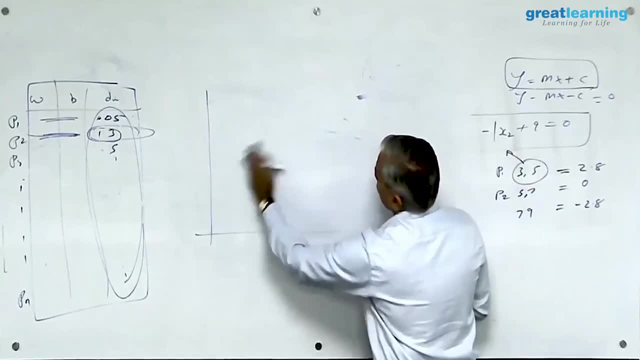 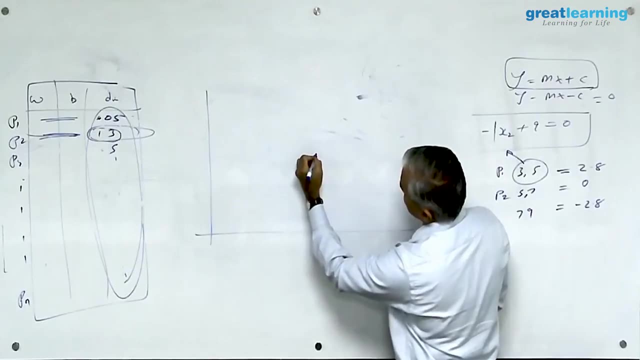 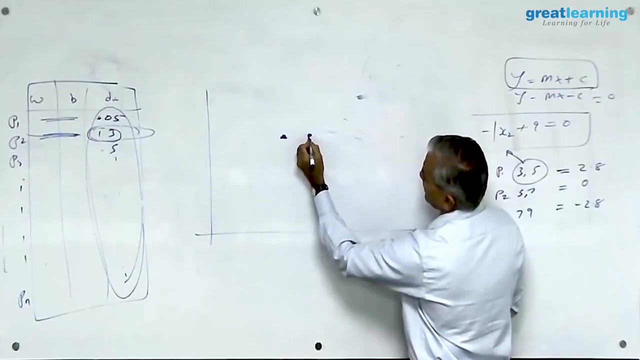 The problem is when I use the magnitude. the problem is suppose there are two points here. How do I show this Just once again? yeah, okay, I can show it this way: Two points from two different classes. let us put this as triangle. this is circle. 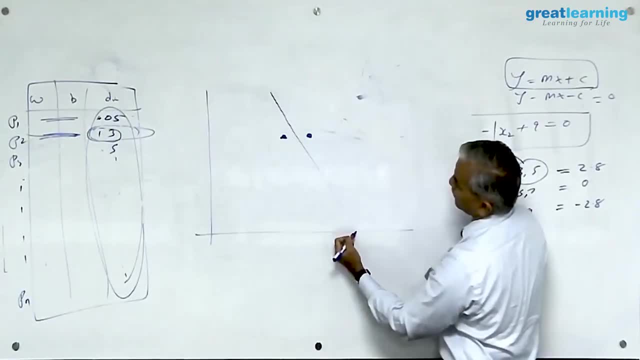 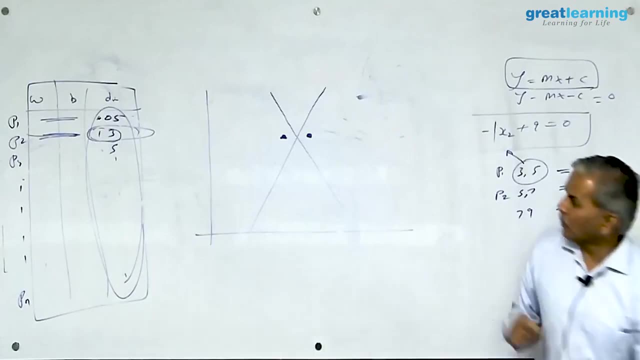 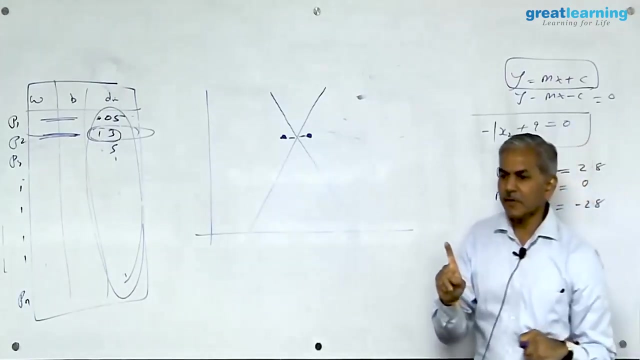 Now you can have two different surfaces: this one and also this one. Both of them are equidistant from this. which one do you take? So when you use modulus, you can end up with multiple surfaces satisfying the condition. Which one do you take? 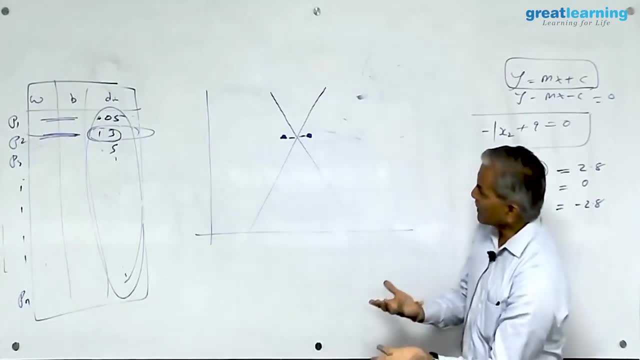 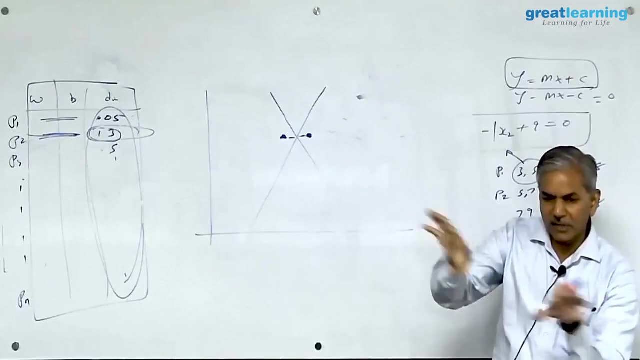 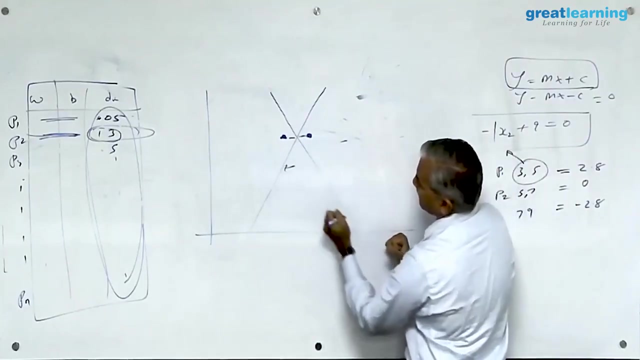 Problem, right, And the other problem is we want all the negative labels to come on the top of the line, positive labels below the line, because we want to give those labels to our classes. So if we use this line, it cleanly separates this as negative, positives. 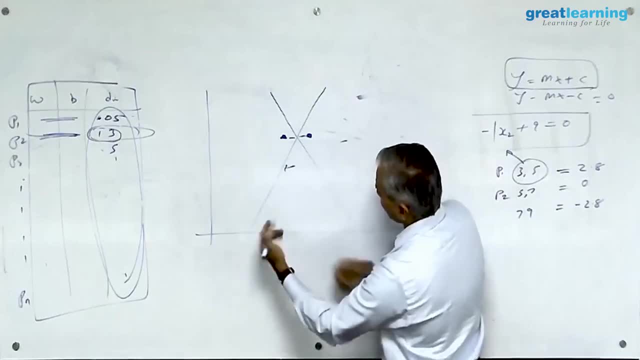 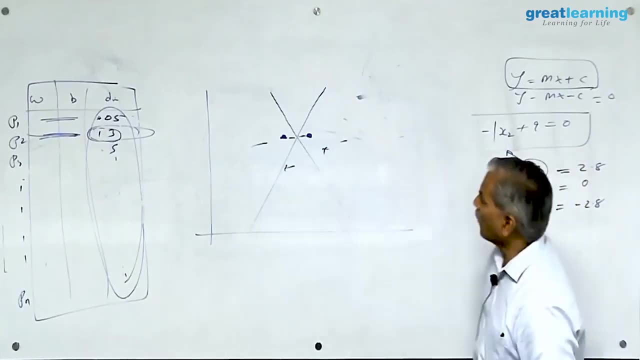 But this line it does the ulta. It incorrectly classifies this as negative, this as negative, this as positive. To take care of this problem, what you do is The distance of any point from this line is given by that. I need my space. 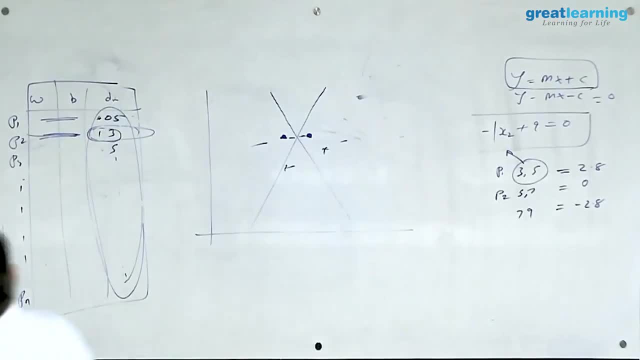 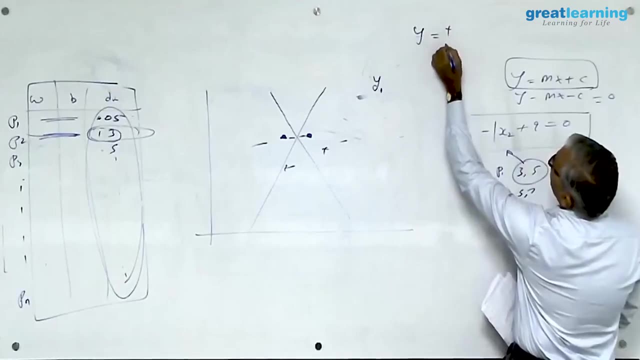 So what we do is we do a simple trick. The trick is we multiply the label. suppose the label is yi label is plus 1 or minus 1, plus or minus, depending on which side of the line you are supposed to be. okay. 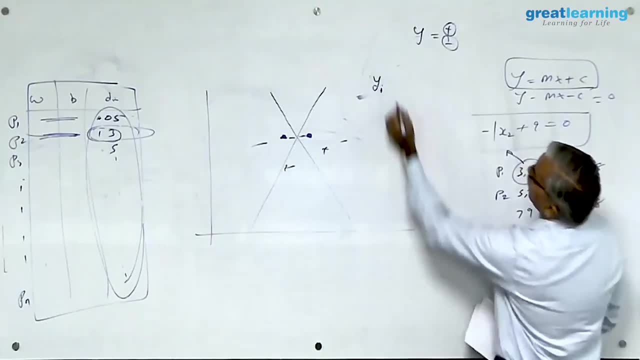 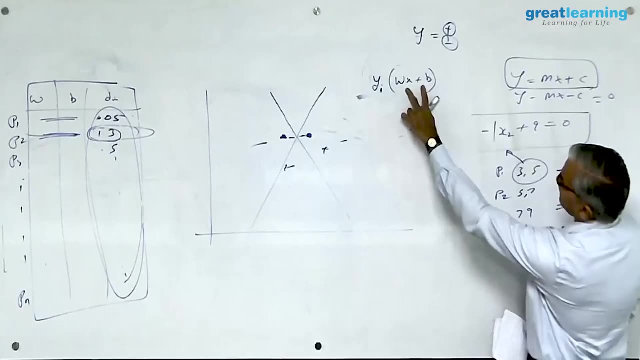 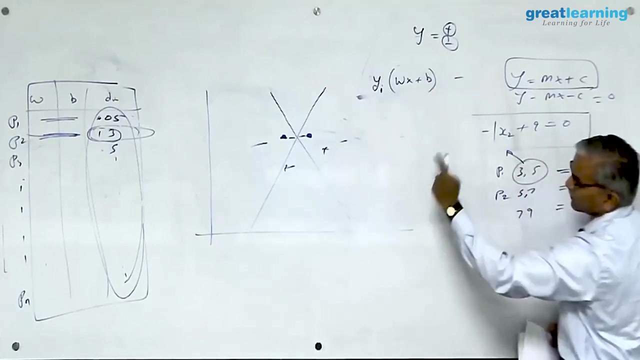 What we do is we multiply the label of the point with the wx Okay Plus b of the point. So suppose wx plus b. when you put this into this equation, it came to minus for the points above the line Okay. 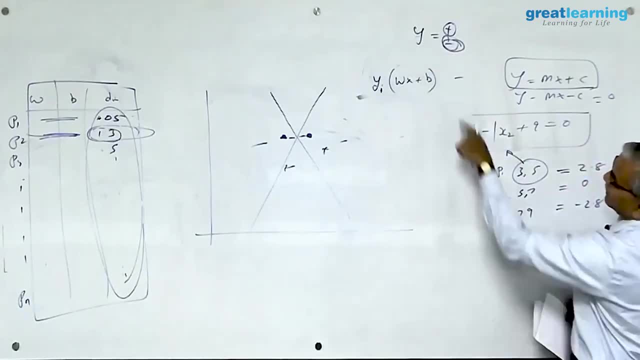 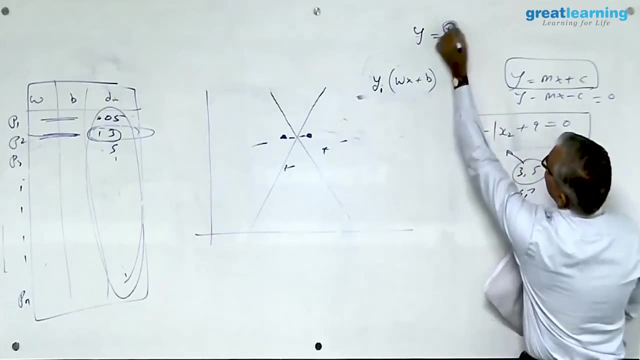 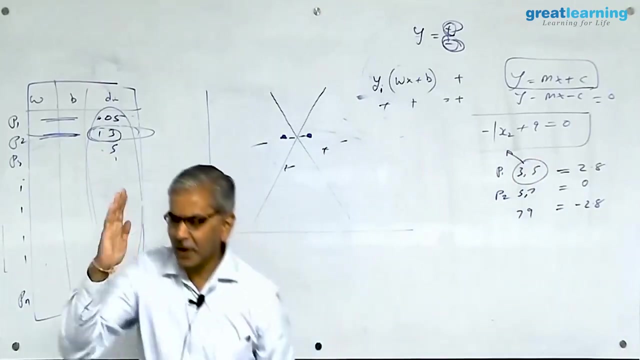 And the points above the line have anyway. symbol is minus, So minus and minus will become plus. Similarly, points below the line: their symbol is plus and their value is also plus. So again the result is plus. Okay, Which means whenever you correctly classify the data points, when you correctly classify, 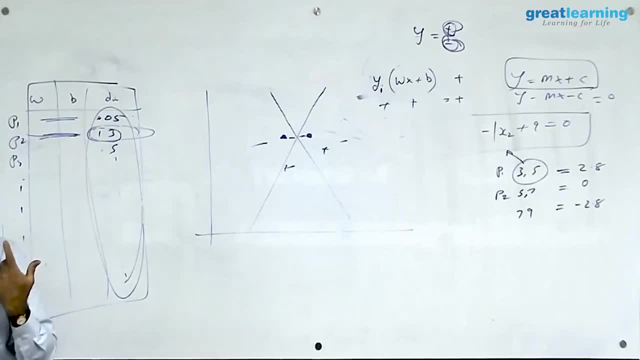 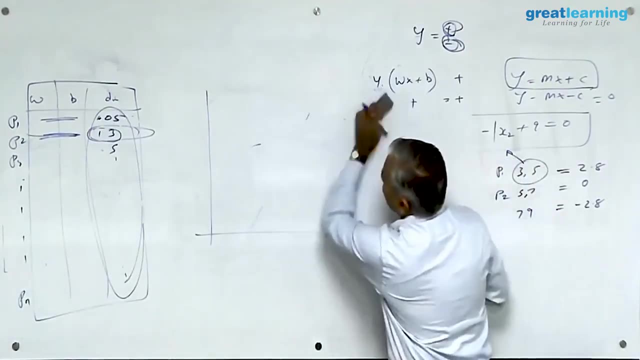 the data points, there are no negative outputs. I repeat again, this is slightly slippery, but it's not rocket science at all. Just look at this. We are assuming that anything above the line- okay, anything above the line- is positive. 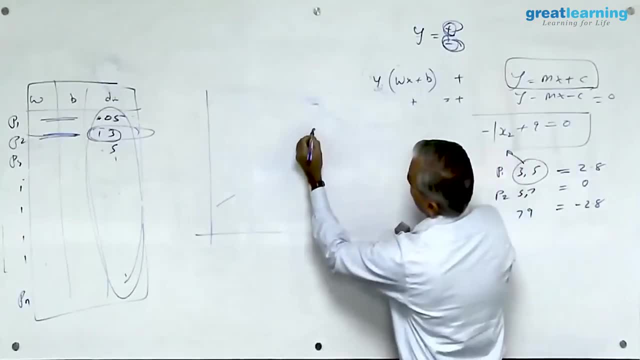 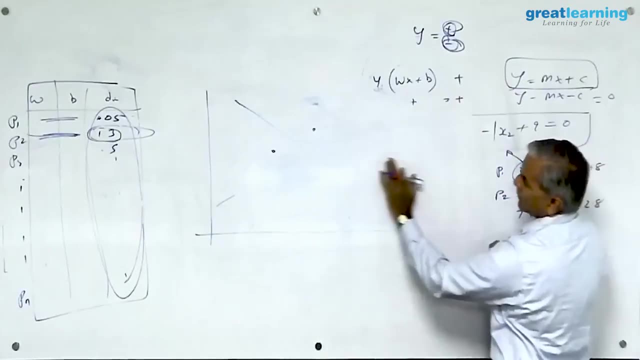 anything below the line is negative. Look at this. I have taken two points from two different classes. This line Okay. This line does the right job. It cleanly classifies. On the other hand, if I put a line, sorry, I'll make it slightly. 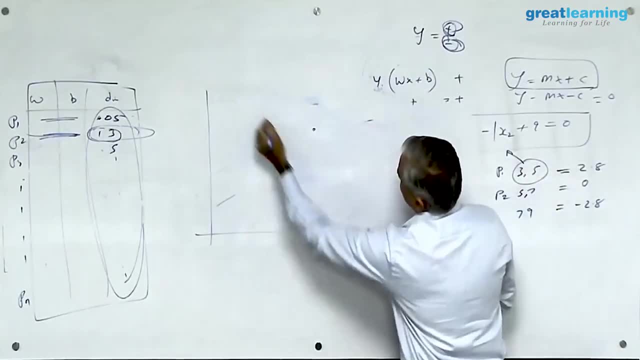 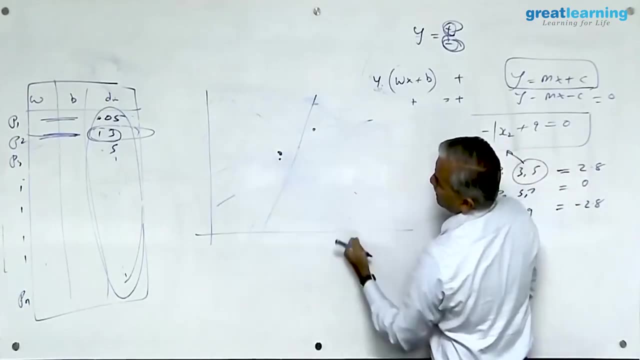 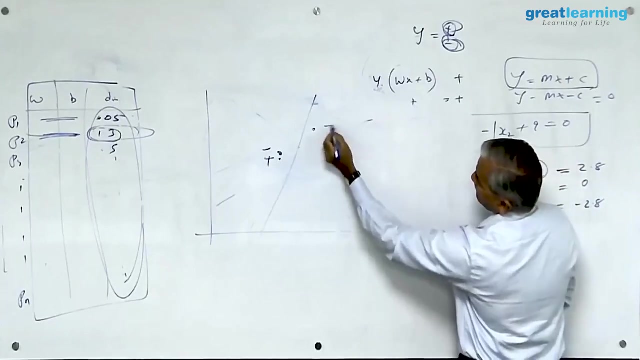 This way. I had this one This way. sorry, This way, If I take this line in this line. this is supposed to be positive number, but because it is above the line, it will be labeled as negative. This is supposed to be negative number. because it is below the line, it will be labeled as: 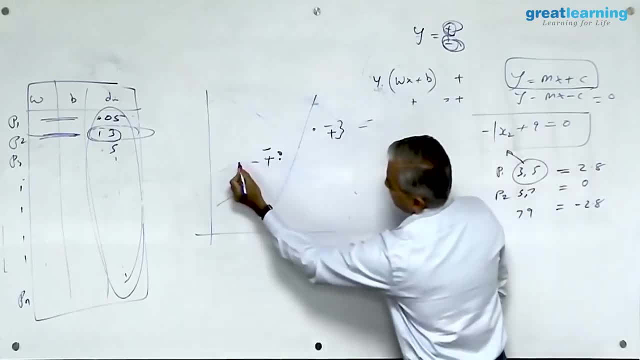 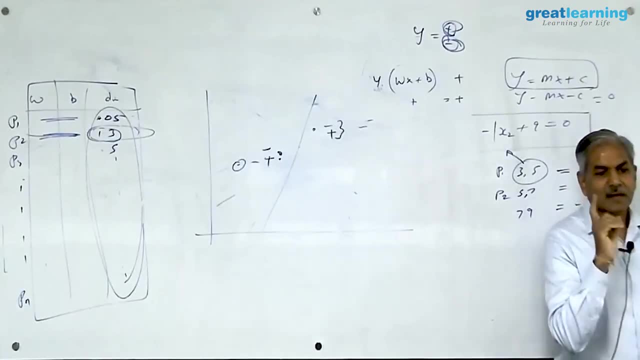 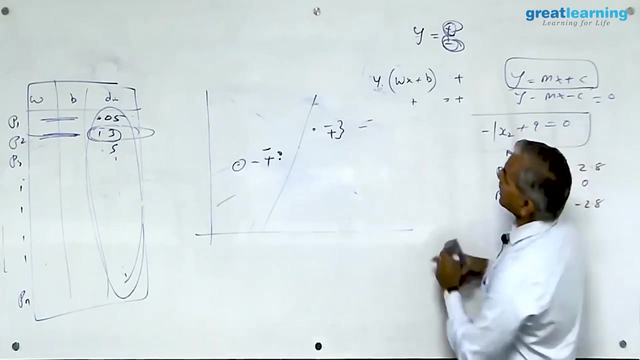 positive. So positive into negative will become negative. This will also be negative Whenever you choose incorrect model. the classifications will all be incorrect and the output will be negative numbers. So the advantage of multiplying this yi, the label with the with, the equation is: 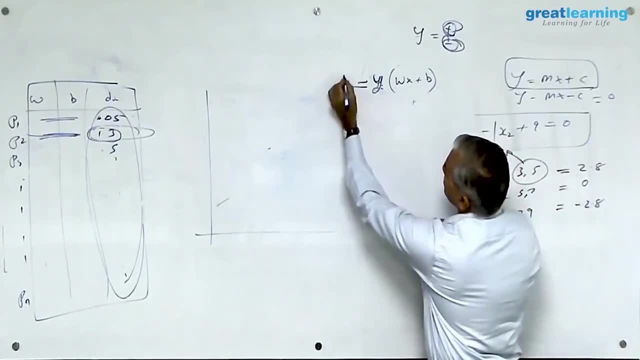 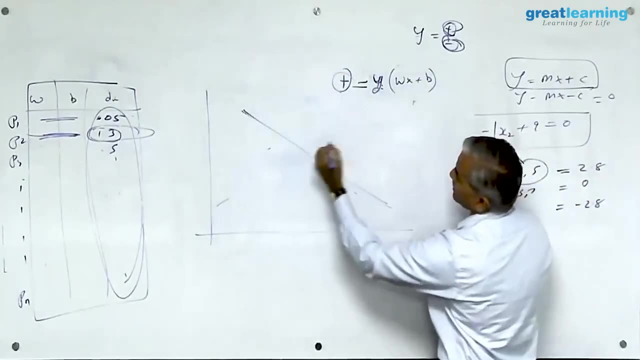 if you get it, get correct classification, this will always result in positive, nothing else. So it will select only that line which gives you the correct result. doesn't matter if there is one more line, it will not select this. 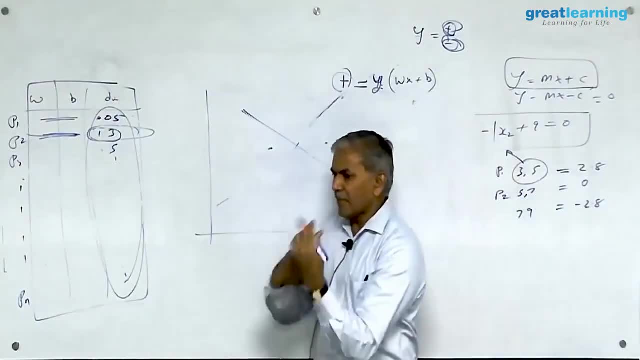 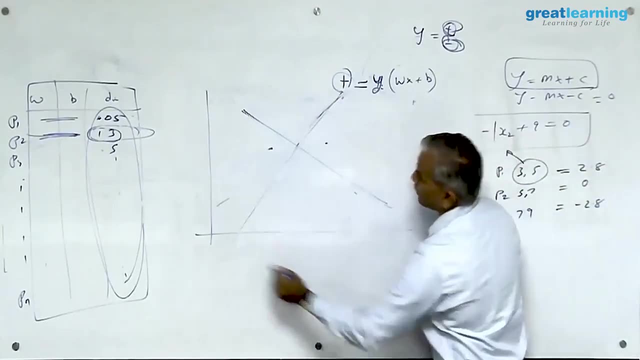 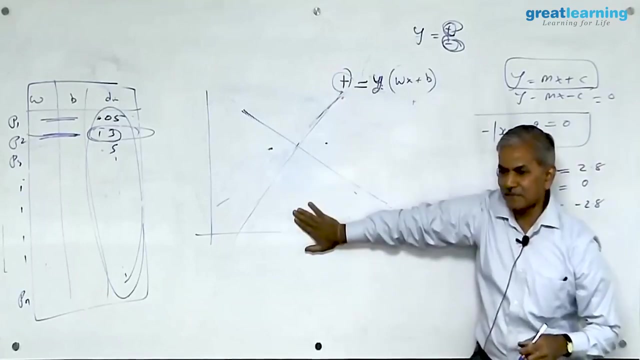 The algorithm will not select this. Keep in mind when we get. when we did a magnitude, we dropped the signs to find the distance. we ended up in a situation where two different planes were possible. This plane will give you everything positive here for both the classes. 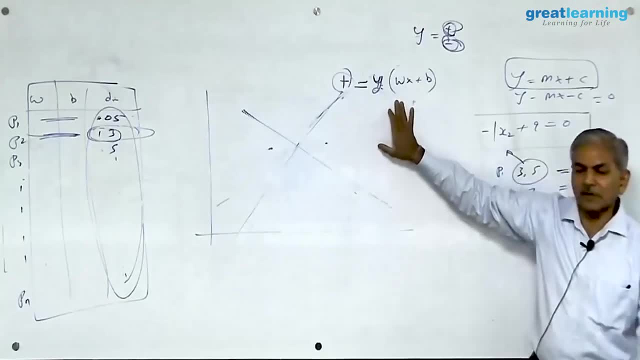 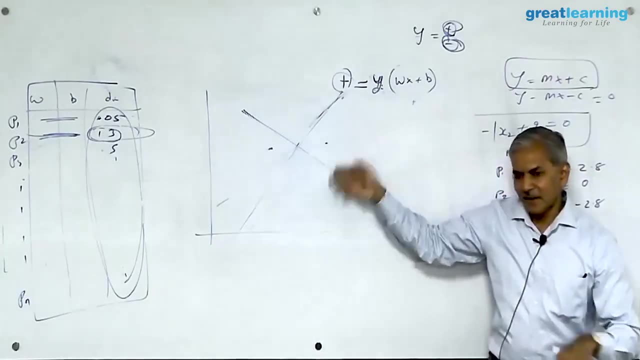 This plane will give you everything negative here. This plane will give you everything positive here. This plane will give you everything negative here. for both the classes, Negative means misclassifications, Positive means no misclassifications, either this side or this side. 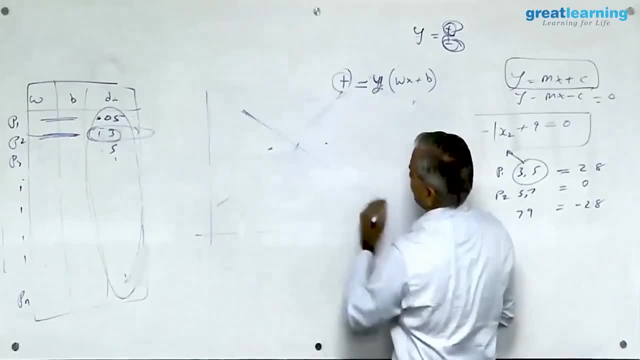 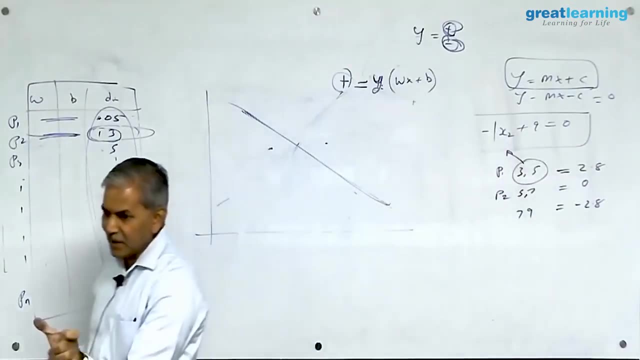 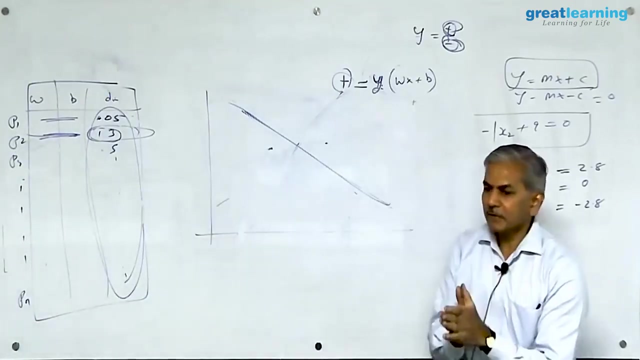 So the algorithm will take not this but this line. So we removed the sign. we removed the sign to overcome the limitation of least with the magnitude. So we removed the sign replaced with magnitude. When we replaced with magnitude, we fell into a trouble where we had multiple planes to 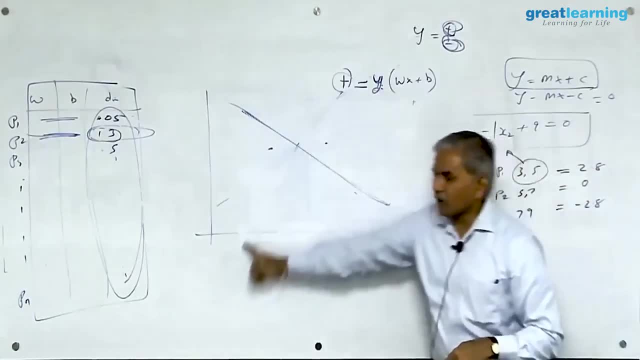 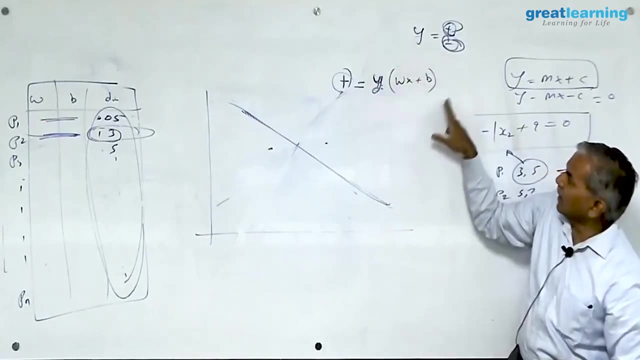 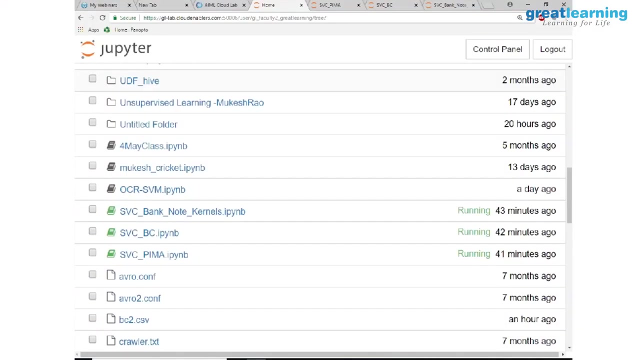 select from One of the planes is wrong. To prevent the algorithm from picking up that plane, what you do is you multiply your equation y and tell the algorithm to pick up the plane which gives you only positive values here- Diabetic allowable minus 1s and non-diabetic allowable, positive 1s. you give the label. 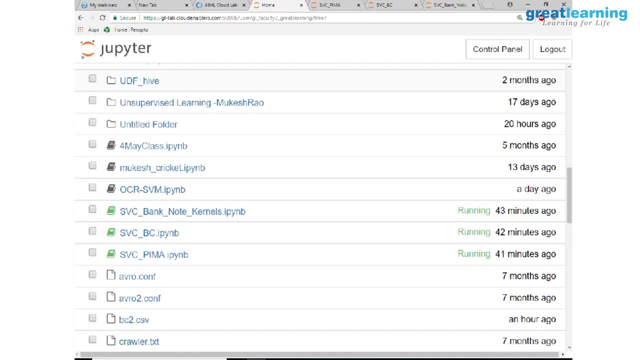 to it. Ok, Now, when you have two surfaces possible, don't worry about above or below. it can be left, right also, right left also. You have two surfaces possible. So you have two surfaces possible In one of the surfaces, you will find that the output when you substitute these points. 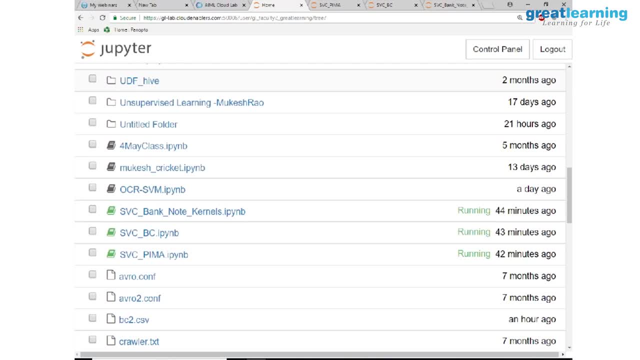 into that equation: the total output will always be negative In the other surface. when you put these points, you see that total output will always be positive, Both the groups put together. whether it is this way or this way, it doesn't matter. 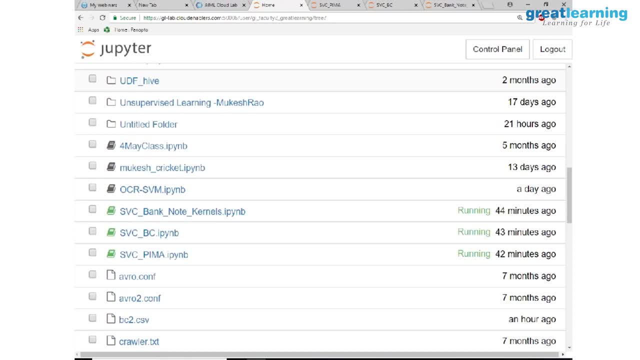 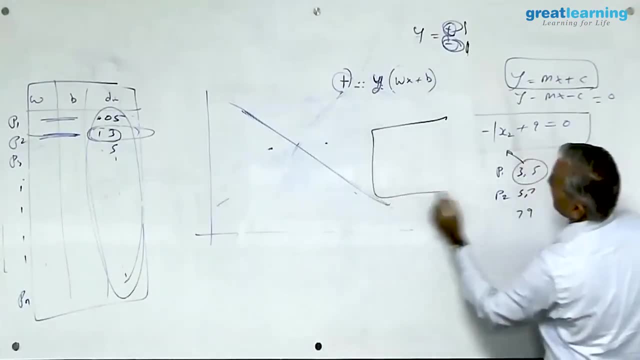 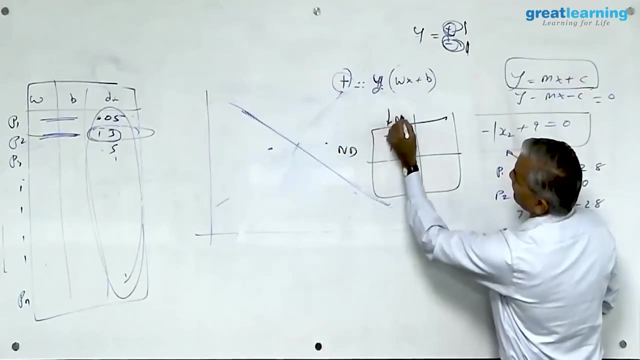 So I pick the line which gives me positive results, indicating that all the minuses have been identified as minuses. all the pluses have been identified as pluses. In the matrix, We had true positives here, right? Those people who are actually non-defaulters have been identified as non-defaulters. 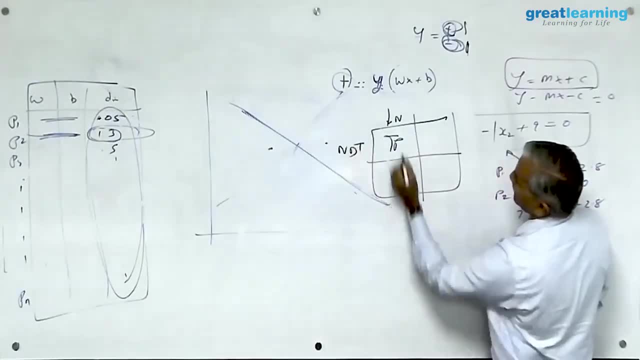 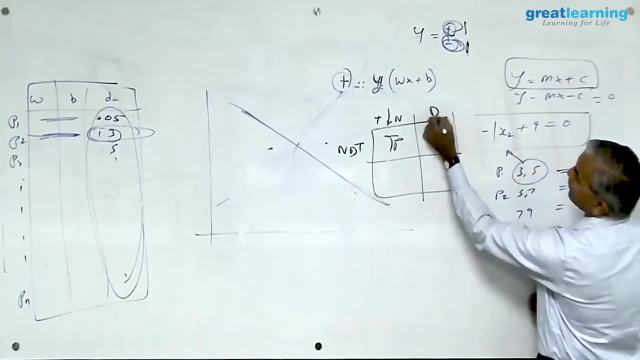 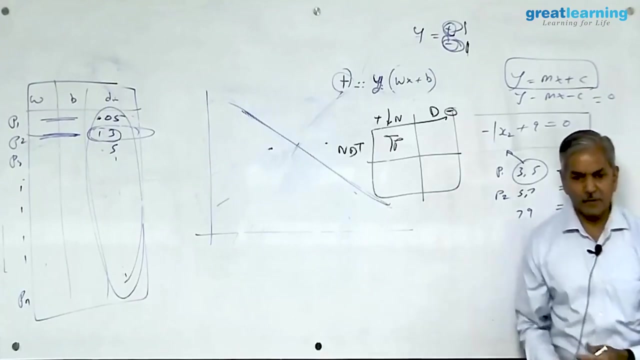 So if non-defaulters have given a symbol of plus, they have been given a symbol of plus by your model also, whereas non-defaulters, who have been identified as defaulters, your model has given them a sign of minus. So what we are discussing in the thing with cross-type, 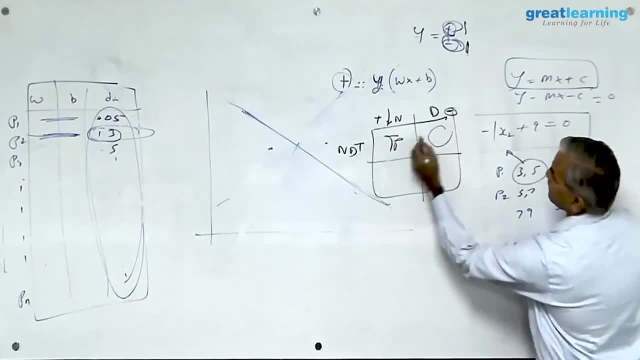 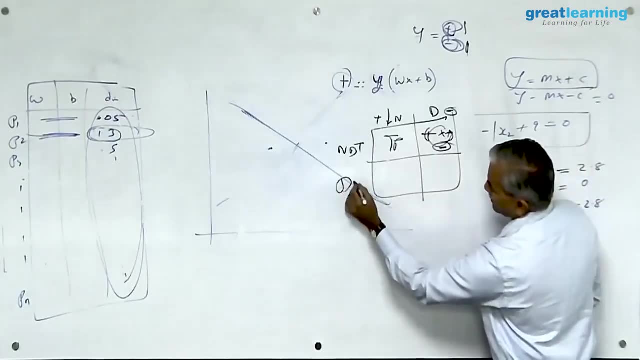 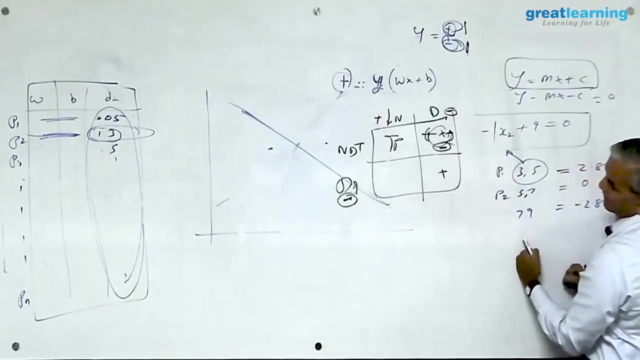 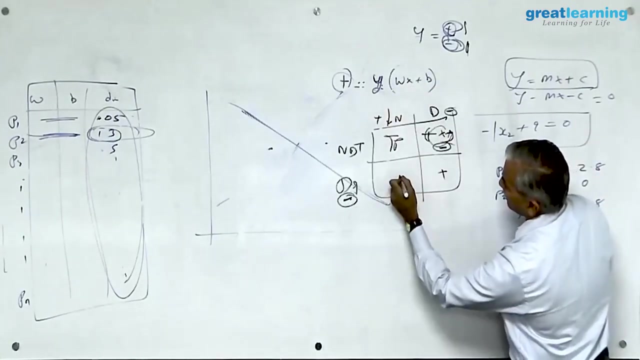 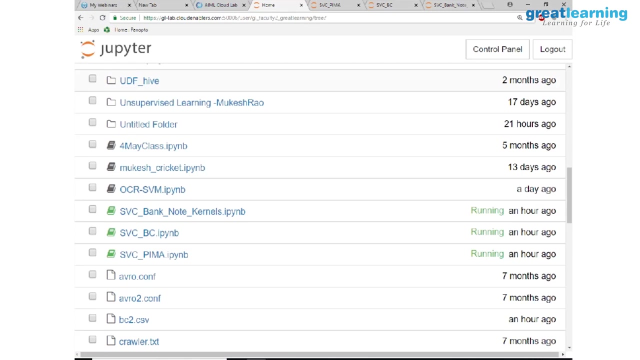